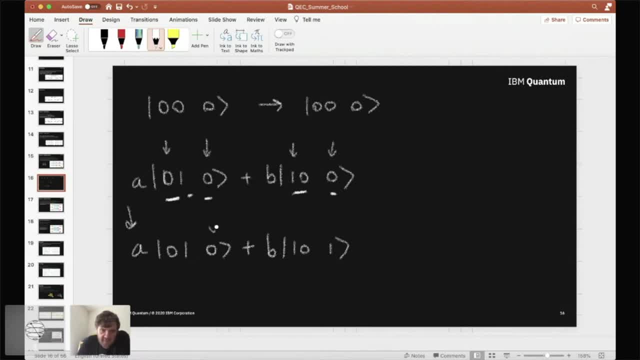 one flips. So now the additional qubit. if we were to measure it at this point, it would be different. It would collapse the superposition, because by becoming zero, it would collapse down to this. By becoming one, it would collapse down to that. 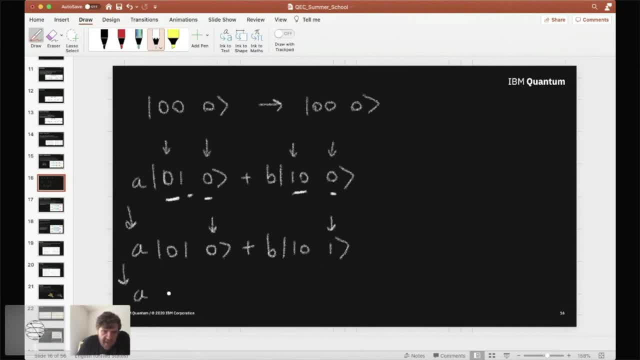 But if we then do the second controlled knot, so zero one, we're now being controlled on this guy here. So the fact that we're controlled on this means that the controlled knot does actually do something. It flips this zero to a one And in the second term, in the superposition. 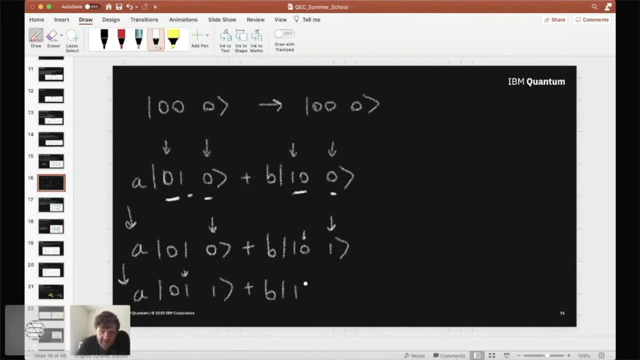 well, again, this is the one that's being controlled. It's a zero, so nothing happens. So this one but remains a one, and then we find in both cases it's a one. so if we measure this, it will give us a one and it will tell us no information about what's. 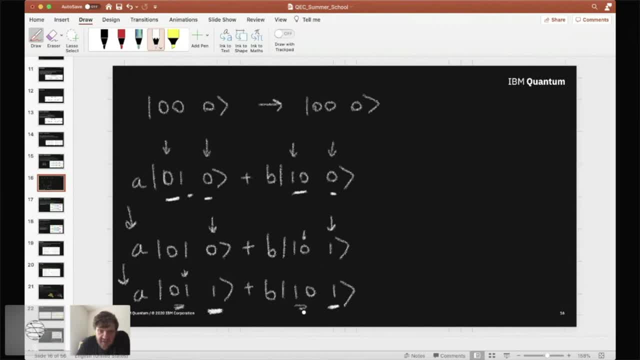 going on and over here, because that it's not even entangled to that anymore. it's completely independent of it. so it just gives us this information without actually changing the superposition. in fact, if we wanted to do some fancy maths, we could basically take that factor out using a tensor product and write this as: 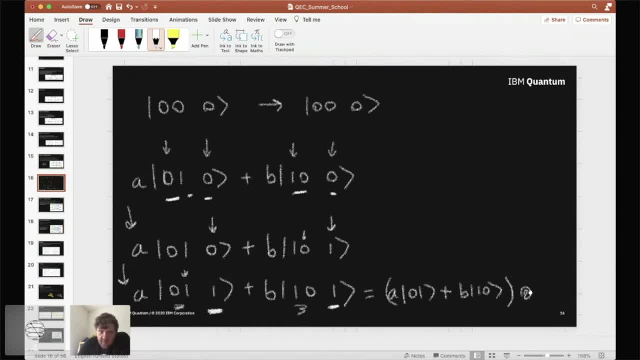 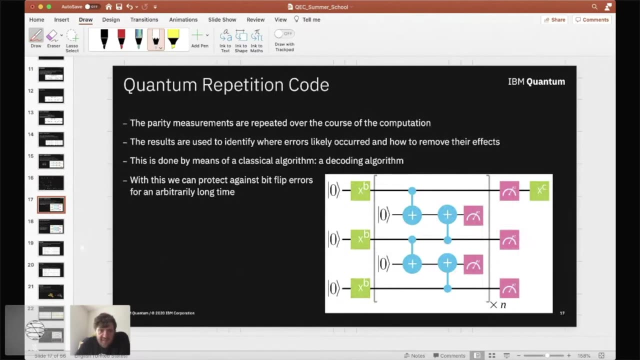 the original state that we had. well, at least if we ignored the additional qubit centered with this one, which is our outcome. okay, so this is our parity measurement. it's it's our syndrome measurement in this form. it's what we do in order to get some trace of error. 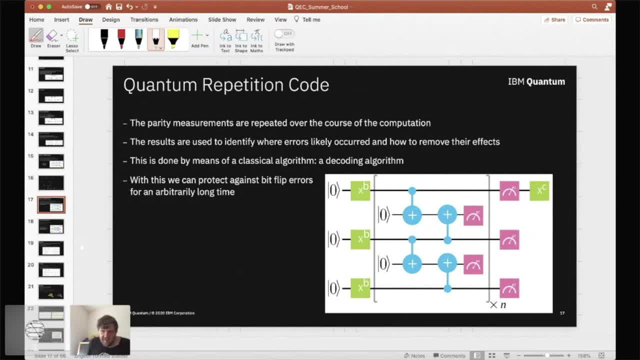 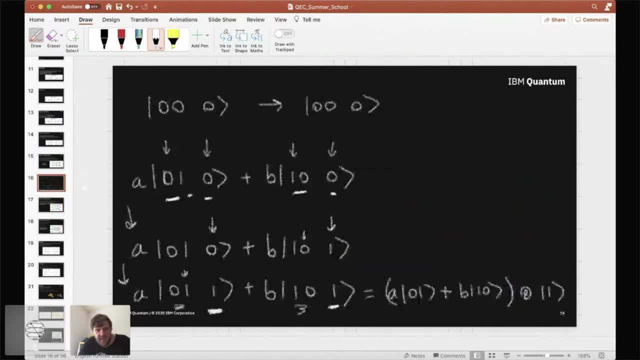 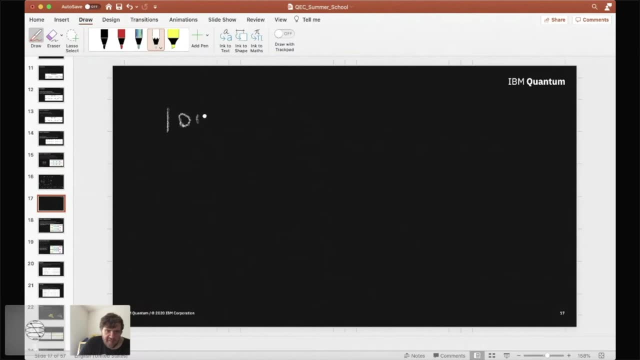 as and errors. I have been assuming so far the errors are just bitflips, which is a very simple form of error. actually, it's more likely that we would get not a bit flip, but something like when we supposed to have say 0, 0, we have a. 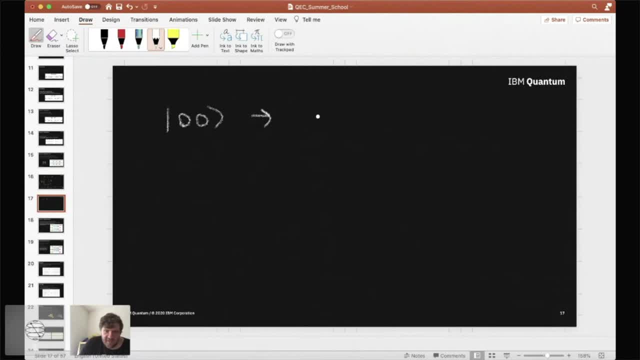 rotation which makes this some sort of- let's say, sine theta zero, zero plus cos theta, beta, 0, 1, and where if theta is 0, then this is close to 0, 0, but some small perturbation of being 1, 1. now, if we were to take this and do one of these parity, 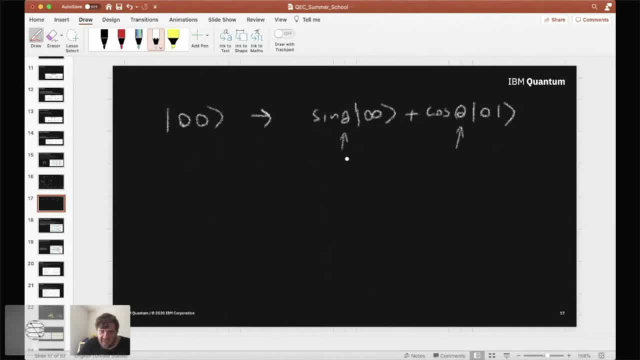 measurements. so introduce another qubit and ask whether it's the same or different. then if it comes out same, it collapses down to this, and if it comes out different, then it collapses down to that. so in this case, this isn't. this is a superposition that's getting collapsed, but it's not a superposition we wanted. 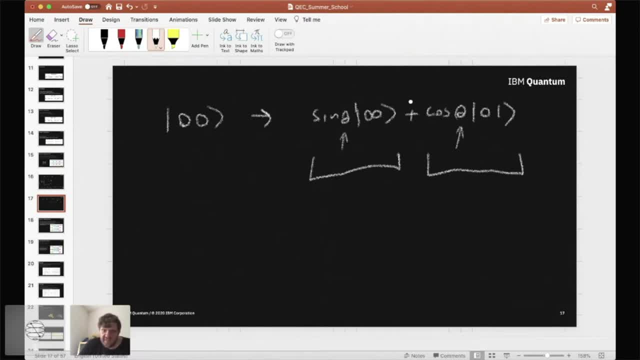 it's not a superposition we care about. so in this case, even though it's, it's a rotation. it's a rotation around the x-axis or the y-axis, it's not. it's not just a bit flip the way that we measure the effects of noise, kind of like. 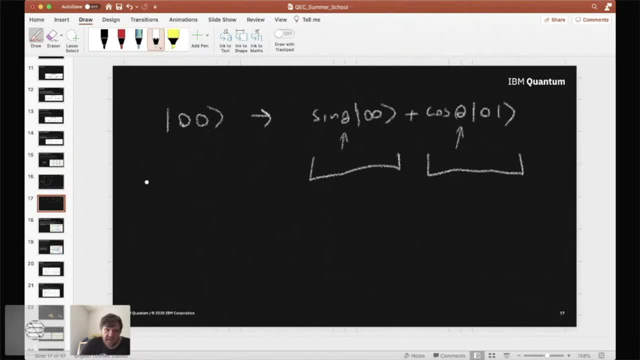 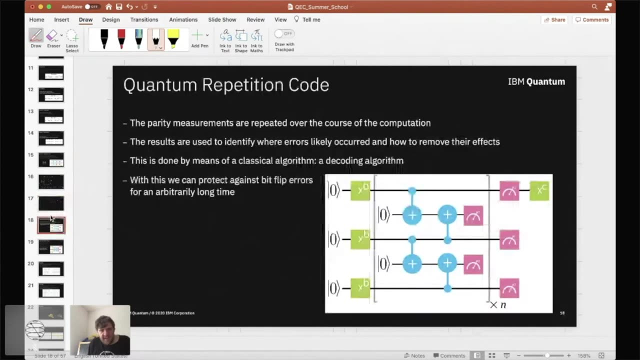 collapses it down to being a simple bit flip. so if, if that went over your head, then just, I'm using bit flips because they're easy and if that made sense and well, good, okay, so we do these parity measurements to get a clue about the errors have happened and the results of. 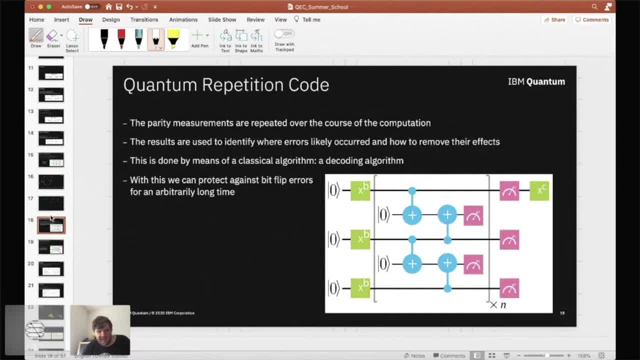 these are used to identify where errors are likely to occur and how to remove their effects, and but to do that, we don't want to do it manually, we don't want to be sitting there looking for all these, these. well listen, this is the same as that, and this is the same as that, and this is the same as. 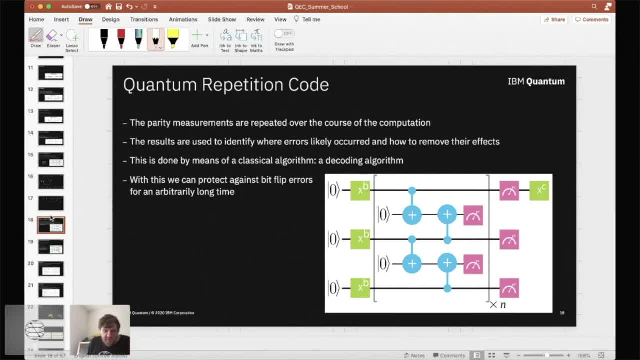 that. so we want to feed these into a computer, a normal computer, and have it figure it out for us. so this process of doing that is called a decoding algorithm. well, it's an algorithm whenever a human does it or a computer does it. but yeah, we usually would use a normal computer to do it and then, once 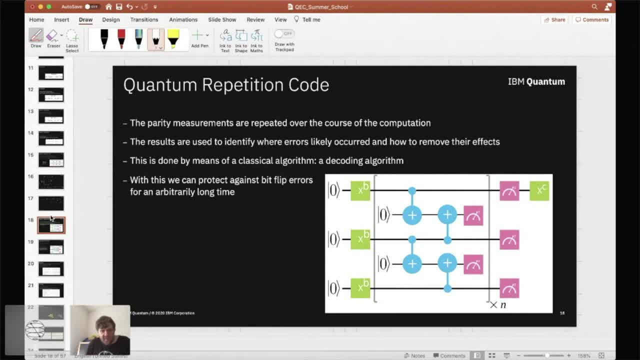 we have this decoding algorithm which takes the information, works out where the errors have occurred and then tries to correct them and protect against simple errors like bit flip errors for an arbitrarily long time, and there is a reason why I'm kind of assuming that it's bit flip errors. 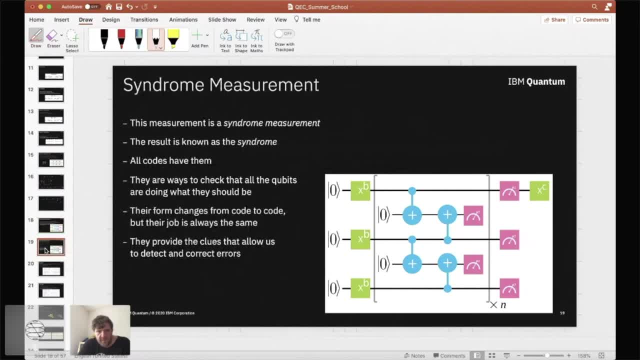 very simplified way at the moment. we'll get on to that later. so, yeah, these measurements, any measurement you do in an error correcting code in order to get some information about the noise, without trying to get any information about the information about what you've actually encoded. so you don't want it when you're. 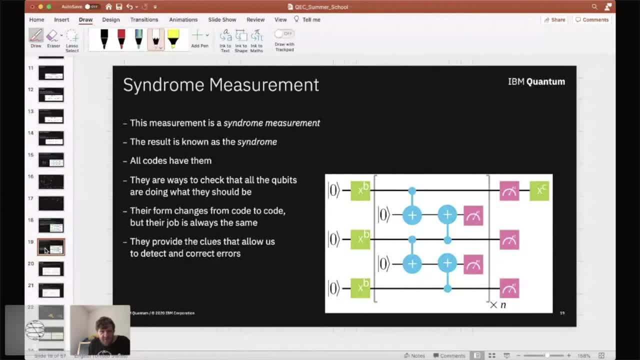 making a measurement which does not tell you anything about your logical qubit. it's not a logical qubit measurement at all. all it's telling you about is noise. that has happened. we call this a syndrome measurement, and the result of the measurement is called the syndrome. so all. 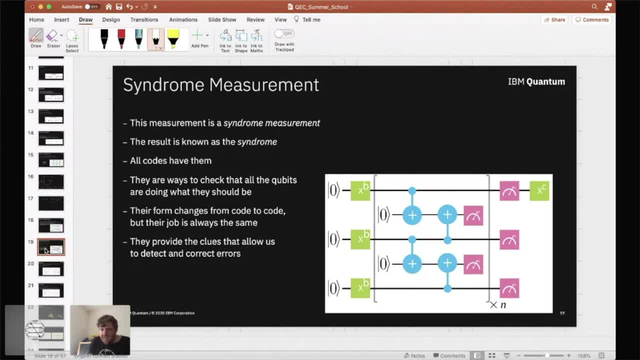 error correcting codes have them, but they differ depending on which error correcting code you are looking at. so in this case they involve two of the qubits of the encoding and- but usually they will involve more than that. you'll be taking a group of qubits in your code and measuring some joint. 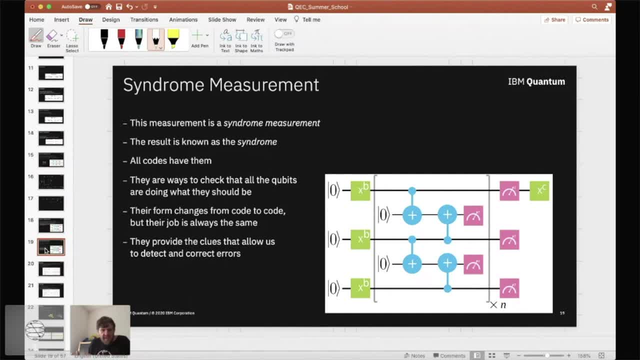 property of those qubits which you know should be something, and you're checking to see if it still is what it should be. so, yeah, they provide the clues that allow us to solve the mystery of where errors have happened and how to correct them. okay, so let's- uh, let's- think more about decoding and to do this, we can start. 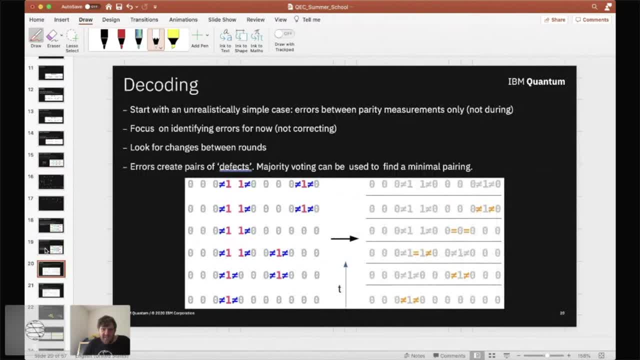 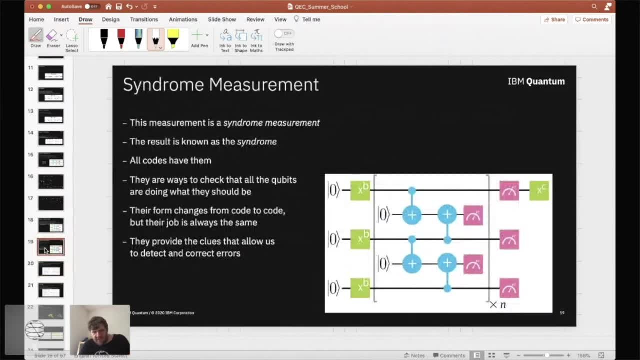 with an unrealistically simple case of a simple error correcting code and we're going to start with an unrealistically simple case of an uh, which is um, that the so always we're. we're getting more complicated in terms of errors, so we're assuming at the moment, 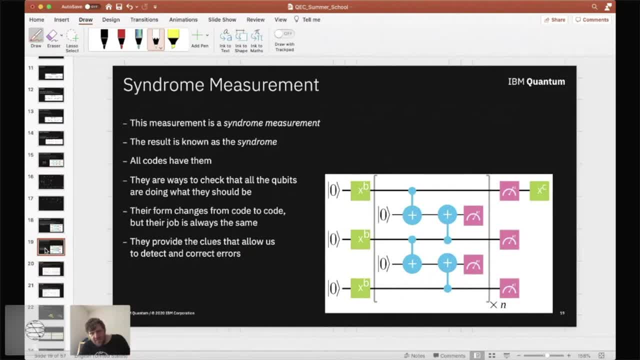 simple bit, flips occurring at very particular points in time, and we're seeing how we can deal with those, and then we we generalize to more complex errors over time. so at the moment we have this circuit where we- well, i should actually explain this a little bit more- we start off with 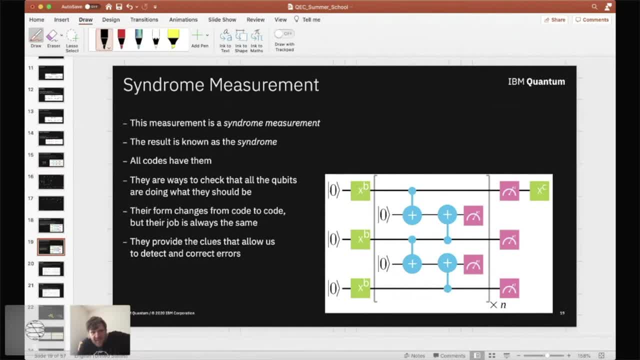 our all zero state. maybe i should make the cursor black again. we start off with our all zero state. um, and if we want to encode a zero, then that's fine. it's already zero repeated many times. if we want to encode a one, it's not fine, we have to use bit flips. 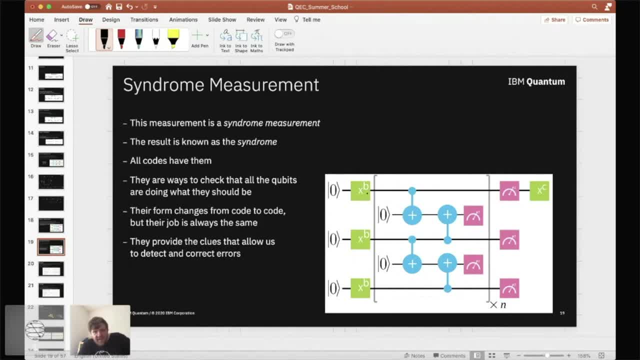 we have to use x gates to flip it. so here, um, we're imagining. this is like an exponent: x to the power of b is doing nothing. x to the power of zero, sorry- is doing nothing. x to the power of one is doing one x. so, in the case that you want to, 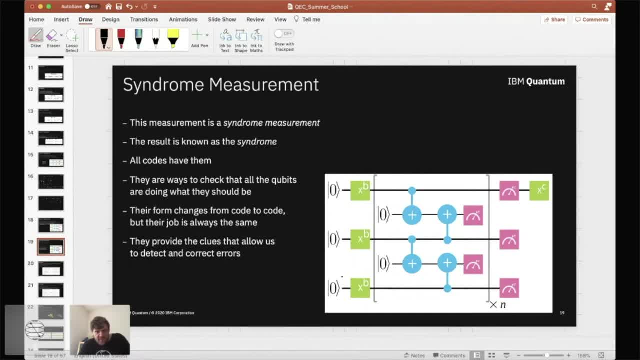 encode your bit value as one, then you'll need to flip these guys to all become ones instead of zeros, and then you repeat this process of checking to see that pairs well, whether they're the same or different, in order to get information about whether noises have happened. and we'll assume at the 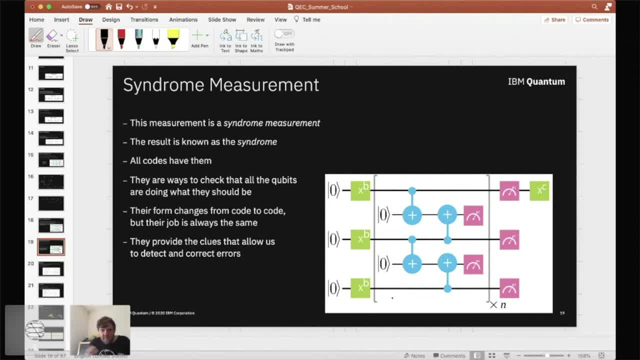 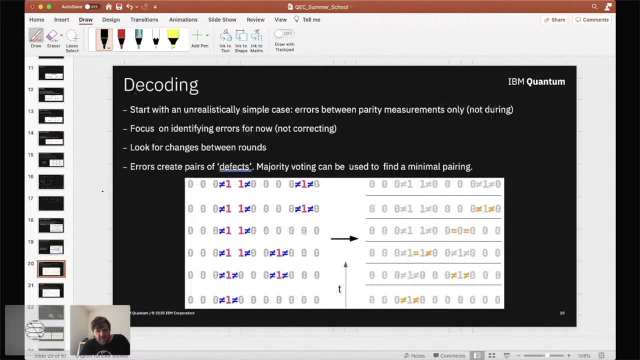 moment that it is between successful implementations of these syndrome measurements that um noise might have a chance of happening. if we take that very simple, um very simple view, then we get quite an easy way of decoding. but it's also a simple form of the more general way of decoding. 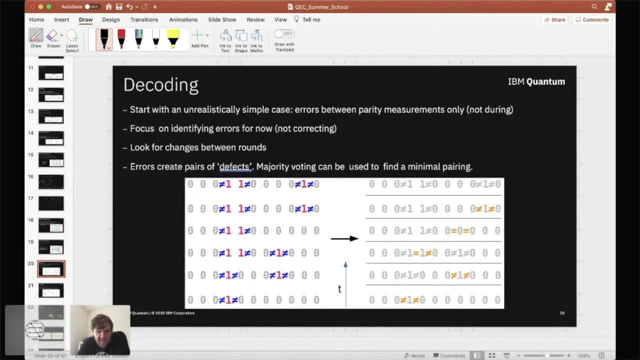 um, so let's focus now just on identifying errors and not trying to correct them. uh, the way we can do this- is the best way to do this- is to look for changes between different measurement rounds. um, so let's see how this works. let's say we have. 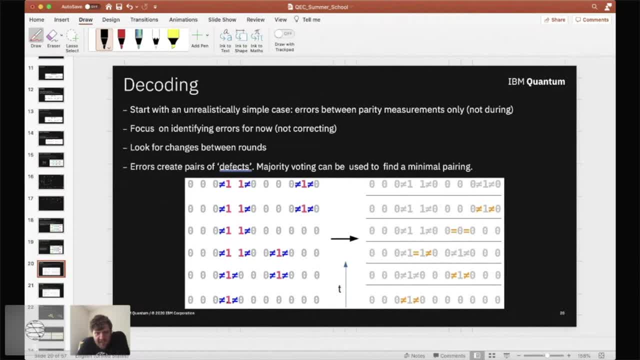 had all zeros and then an error happened here and gave us a one. it doesn't actually matter whether they're zeros or ones, it just matters where the errors are happening. and then our syndrome measurements we're making tell us that these two are not the same. they 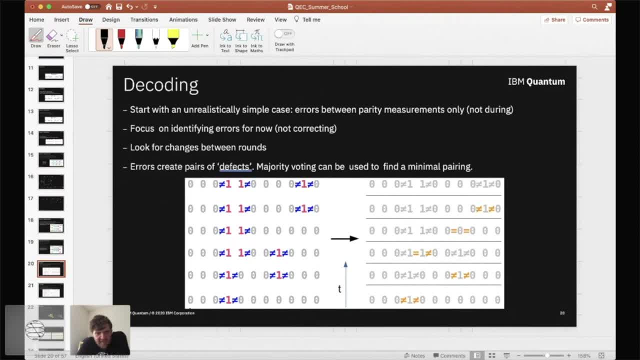 tell we, may we measure the syndrome for these two? and it tells us: same we measure it for these two, same we measure it for these two. it tells us that they are different. for these two, different, same, same, same, and so on, um, so we see some trace of errors here, the fact that these are different. 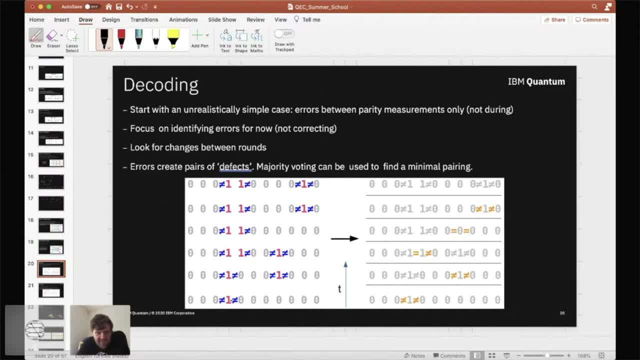 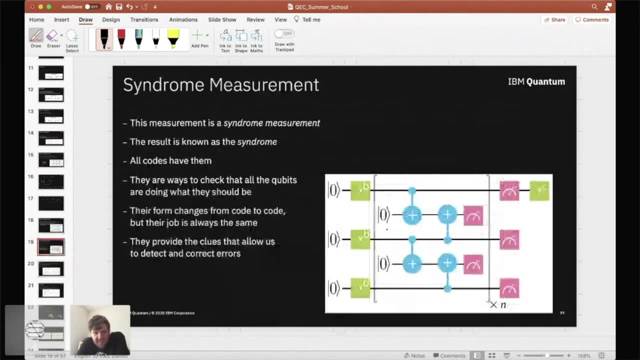 from each other. this pair, these are different from each other and these are different from each other- is a signature. then error has happened here. now we so that round of measurements is complete. then we start because we're constantly repeating this, we're constantly repeating these measurements. so we then do the next round of measurements. well, what do we find? 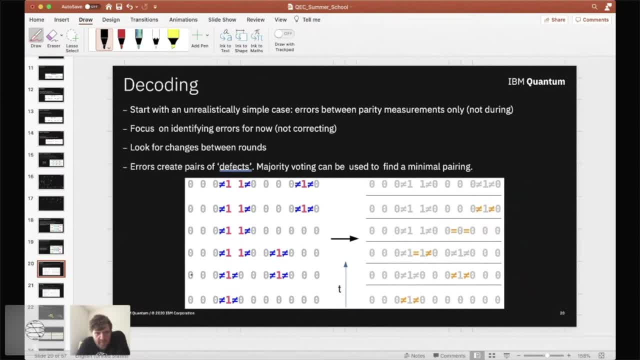 well, we would expect that these will be the same because, um, that's how we set them up in the beginning and they were still like that last time. so we expect them to still be like that, and we expect these to be the same, because that's how we set them up at the beginning and that's what they were last. 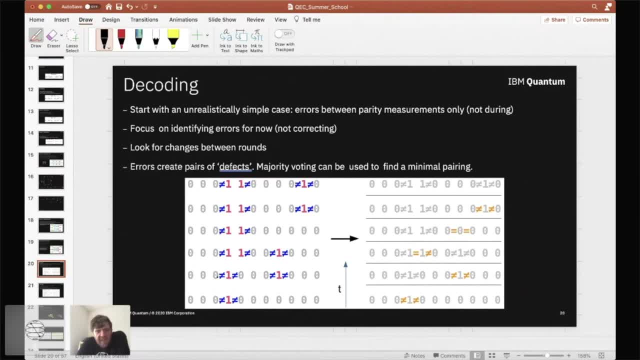 time. so we expect them to still be like that and we expect these two to be different? uh, because even though we set them up to be say the same at the beginning, we we measured that they were different last time and we haven't expected that error yet. we've just logged that, it's there, and so we still. 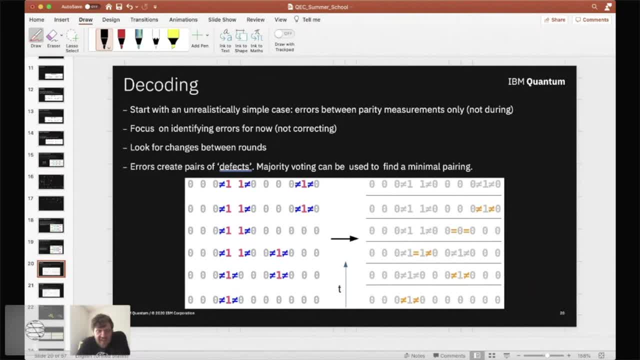 expect it to be there. so the fact that these are different in this measurement round is not a signature of error. it's a signature of things being the same as they were. it was a signature of error when we first saw it, but it's not a signature of error. 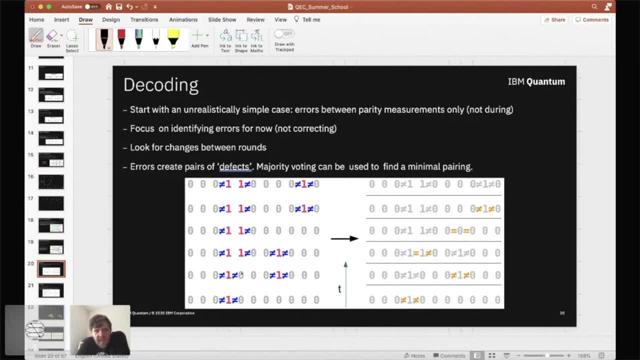 anymore. it's old news, it's expected, whatever. and still, these are the same, that's fine. these are the same, that's fine. these are different. well, that's new. we haven't seen that before. so that is a signature of error, as it is, for when we see that these are. 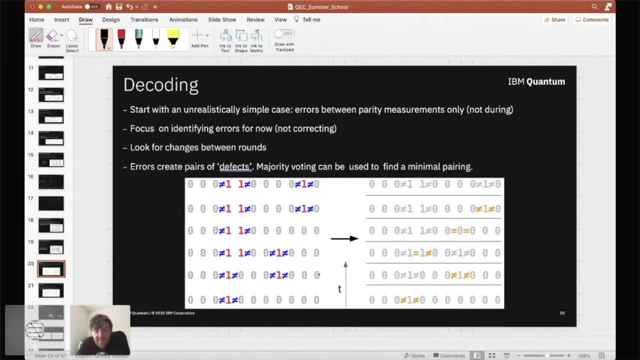 different. uh, these are the same, these are the same. so from this we can see that what is the the good thing to do is actually to track um differences. so when we find things that we don't expect, so here, when we find these differences that we don't expect, then we say, okay, this is something. this. 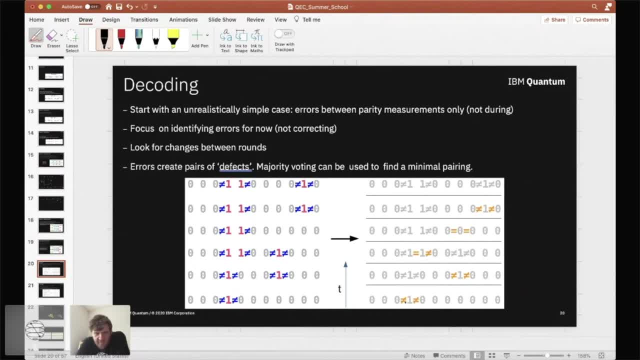 is a significant event. let us log these two times that we saw something that we didn't expect, when we, when we saw the same result again- well, who cares? so we don't log that. um, but over here, when we're seeing this for the first time, that's significant, so let's log that. 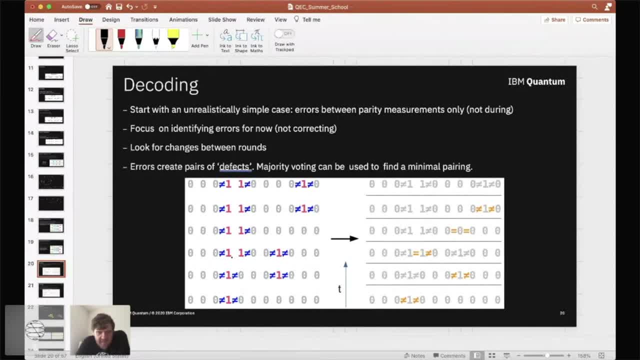 now. an interesting case in it over here is when, um, another error happens right next to the error that happened before. so now when we ask these two, are you the same or different? they say they're the same, and then usually you think being the same is a good thing, right, because that's how we set them all up at. 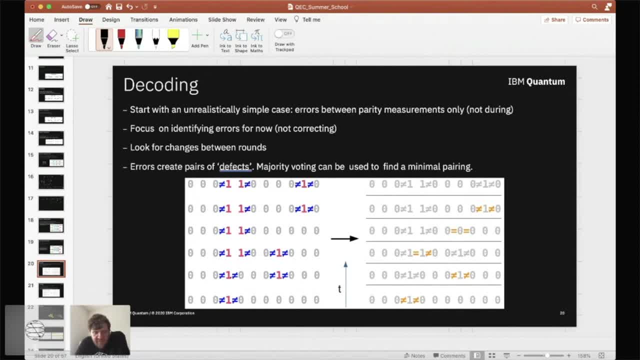 the beginning, but since we have already previously seen them to be different, this is a change. something has changed this. something has changed these values and we have- we aren't going around changing these values, so it's a signature that an error has happened. similarly, when we see that these are: 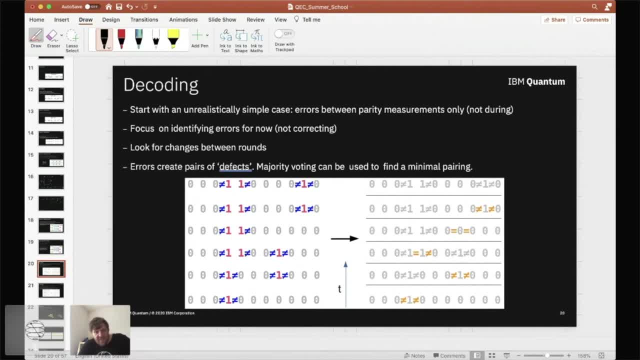 different, then that is also a signature, that is something new. that's a signature that an error has happened. so we log these two things, even though these are the same. it's a signature of something changing, it's significant, we log, and so we go on looking at all these. 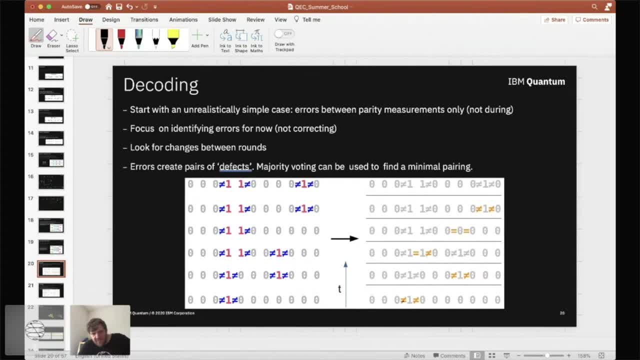 syndrome changes. what we find is that when we look at the syndrome changes, they always occur in pairs and in these cases only one little error is happening at a time, so these pairs are fairly close to each other. so if we look at this, it's fairly easy to see. 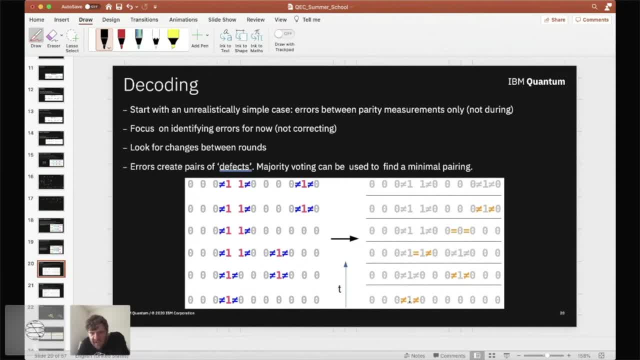 okay, we've got a pair of syndrome changes here. there's probably an error here. we've got a pair here- there was probably an error here. a pair here- error here. pair here- error here. pair here- error here. um, so with this we can figure out where the errors most likely happen, and this is a very simple example, but we 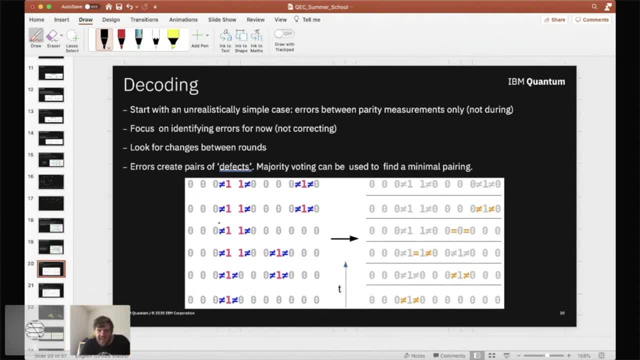 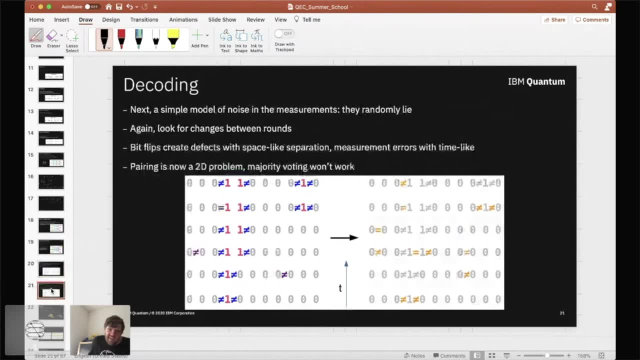 don't really need an algorithm to do this, we can see it by eye, but nevertheless, um, well, there you go. um, now let's uh, introduce something more realistic. so, uh, for example, what if, when we made the syndrome measurements there were, they didn't. they didn't happen perfectly. 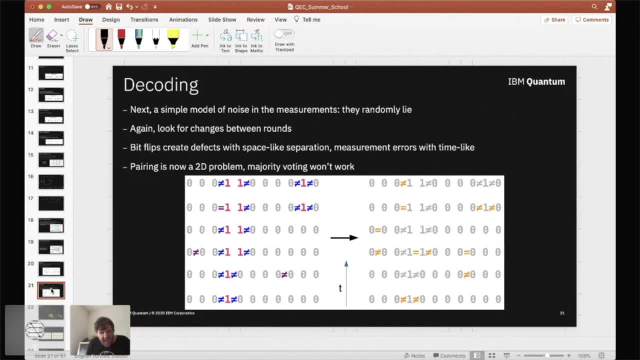 so before we've been assuming that when we make these syndrome measurements they happen perfectly, and then between different rounds of syndrome measurements errors can happen. well, let's assume now that the syndrome measurements do not happen perfectly, but some things can happen, some things can go wrong with them. so as a very simple model, we'll just 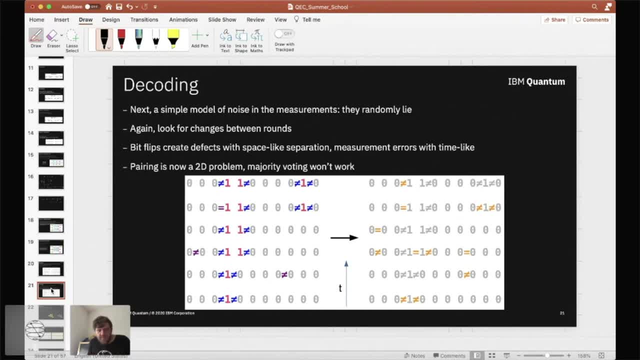 assume that sometimes they lie. sometimes, when they should tell us zero, they tell us one, and sometimes, when they should tell us one, they tell us zero. there's no actual change on the qubits. uh, they're just lying to us. uh, so if we take the same sort of thing as before, but we introduce some of these, 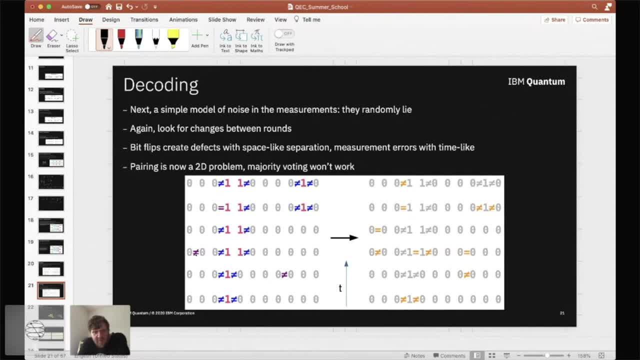 lie, errors. well then, maybe here, um, we saw that these two, we asked: are these two the same or different? and it said: they're different. and we, and we take, we, we, we believe them, um, but let's suppose that this, in this case, it's a lie. so then the next case, when we look at the 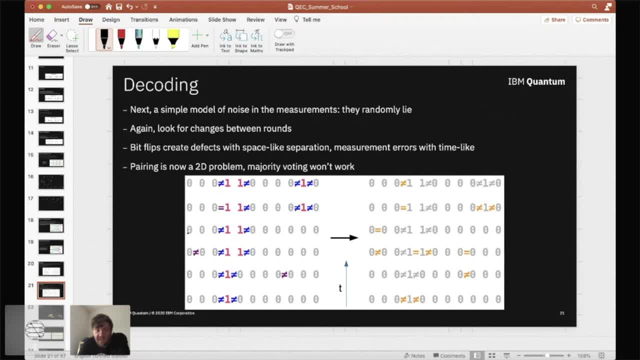 whether they're the same or different. we see that they are the same and then we're like what i thought they were supposed to be different. so when we saw that they were different, expecting them to be the same, that was a change in the value. that was something unexpected. 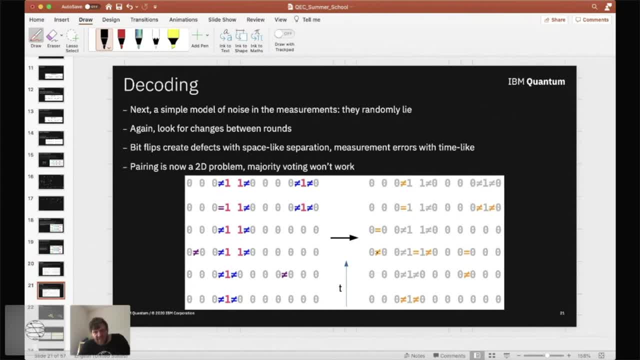 and so we logged that. but then when they returned back to saying that they were the same because they, because the measurements- stopped lying, that's also something significant. so now, even in this case, where it's completely different type of error, we're seeing that an error is causing a. 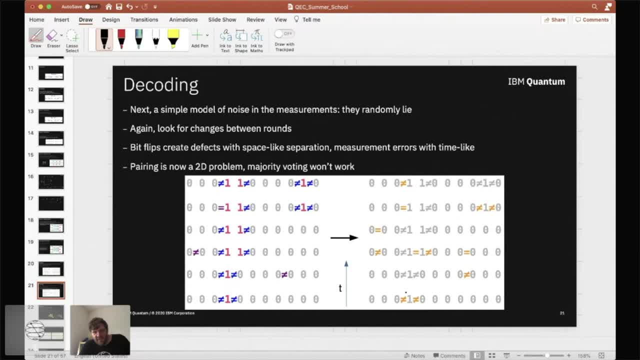 pair of these syndrome changes, but, rather than being what we might call spatially located, we cut different places along the line because of an error that's flipping a bit. uh, they are what we might call temporarily located. they're on in different measurement rounds, but they're still pairs, and so we can still go through this and say okay. 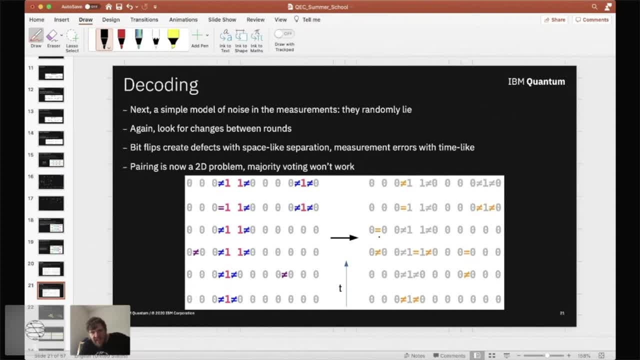 that's a. that's probably an error here. uh, this is probably a signature that there's been. one of the measurement outcomes was lying to us and so we can go through this and so on and so forth. so now, um, still we we're going around identifying pairs of these. 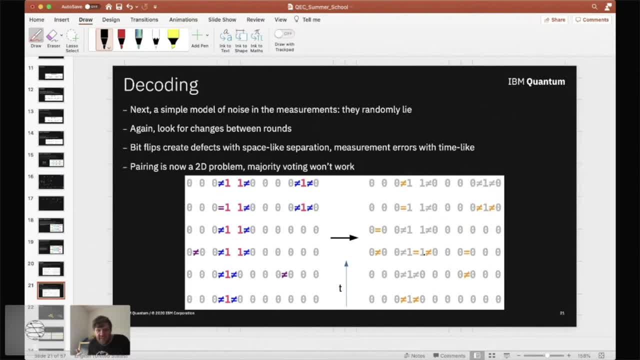 these values, that where they are what they're, not what they should have been, uh, but the we have to identify the pairing. but the pairing is now effectively a two-dimensional problem. it doesn't, it doesn't correspond to majority voting anymore. it's a more abstract, uh problem of. 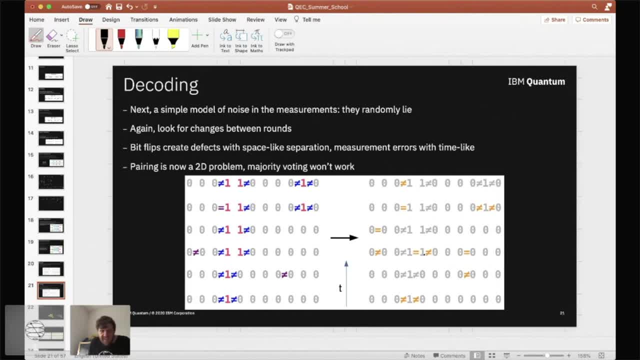 trying to work out where the errors have happened, and this is, even if you're adding- you add in now- every different kind of error that could possibly happen, it still remains like this. so, uh, we now basically, by finding pairs of measurement results that aren't doing what we expect them to do, 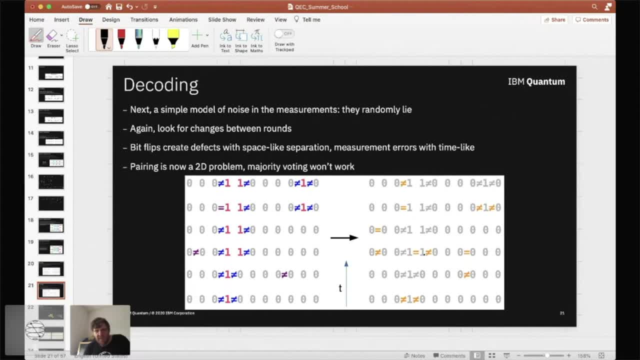 we can deduce what how to correct. now i don't i think i'm going to go into full details about about this um, but this should give you enough get a sense of decoding. And, of course, I made this Dekodoku game a few years ago. 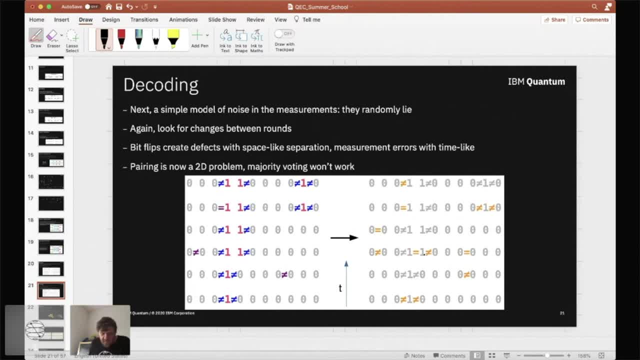 as a way for you to really get hands-on experience. So that's something also that you can try out if you like. We really should make an IBM version. So, OK, I think at this point I should maybe ask if there's any questions. 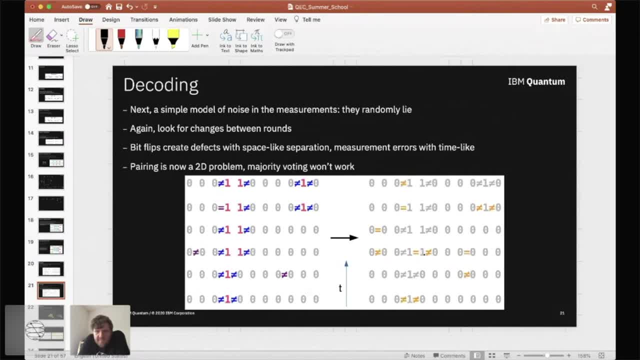 So good news. we have tons of questions. I just want to remind everyone that we're not going to be able to get to every question here during lecture, So remember to bring those questions with you to Discord, post them there or anywhere else. 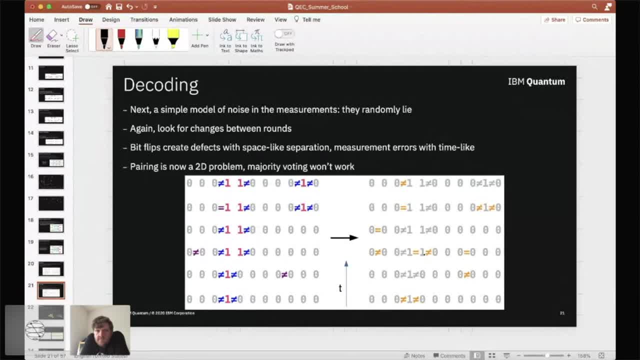 And talk to each other about them. But our highest-uploaded question- you've kind of already touched on it, but just want to put a formal question: What effect does repetition code have on the speed of an algorithm? That's a hot, dead-diver question. 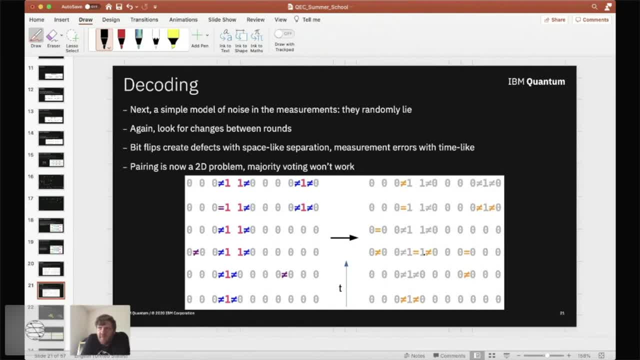 It's an interesting question. So well, the repetition code has issues that makes it not so useful. So probably you wouldn't use a repetition code in an algorithm. So instead I'm going to say just in general, for quantum error correction, what effect. 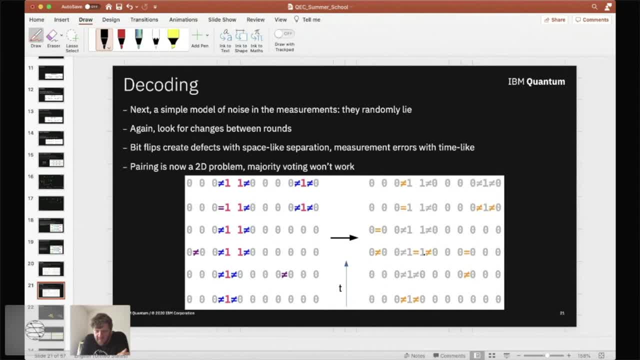 does quantum error correction have on the speed of an algorithm, And it very much depends on what error-correcting code you're using. So there is a need- and I'll touch on this more later- to be able to do So when you have a logical qubit which 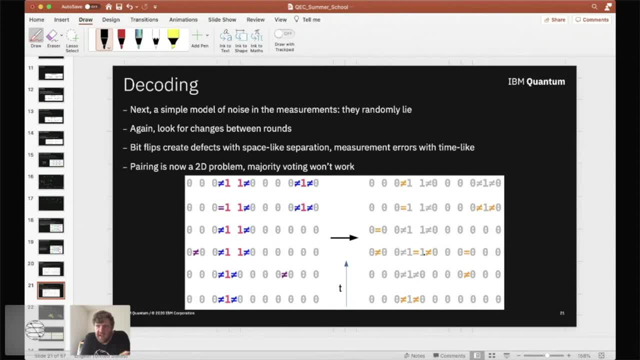 is spread across many physical qubits, you have to do gates on those. You have to do your gates on your physical qubits. That involves doing gates on many logical qubits And if you can find a code in which doing those gates is what we call transversal, so you can do them in a single step. 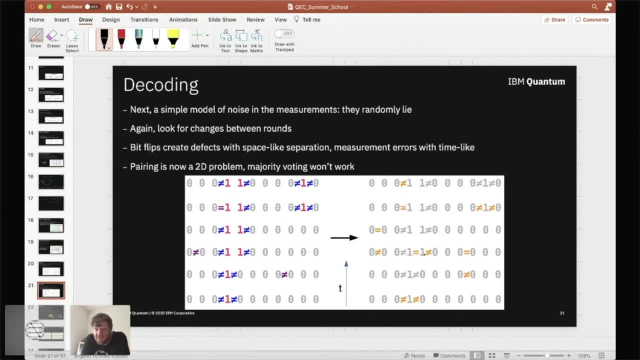 you can just do a whole bunch of things across your encoded qubits And you can do a single logical operation, Then it wouldn't- in terms of it doesn't- really affect your algorithm runtime all that much. There would be some factor that you 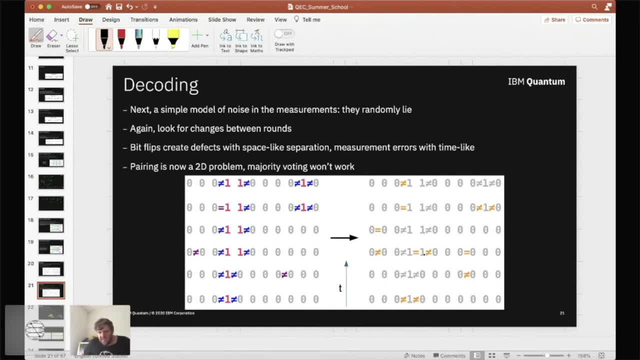 would have to take into account, but it wouldn't affect it all that much. But the trouble is that there are some operations that are very hard to do within an error-corrected way, And so, for example, just a single qubit rotation. 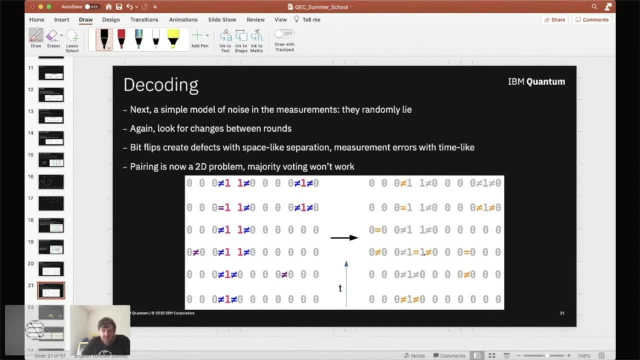 it's something that is usually really hard to do And you have to devote quite a lot of resources towards doing a single qubit rotation- Things like control not to be very easy, but a single qubit rotation is hard, So you would need to do your circuit would be a lot bigger. 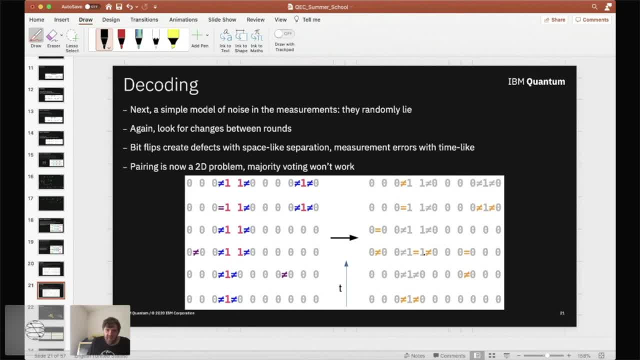 It would have a lot more qubits, It would take a lot more time than it would if you didn't use error correction, But it would work at the end, which is the important thing, Cool. And another question: Can the repetition of our answer either yes or no? 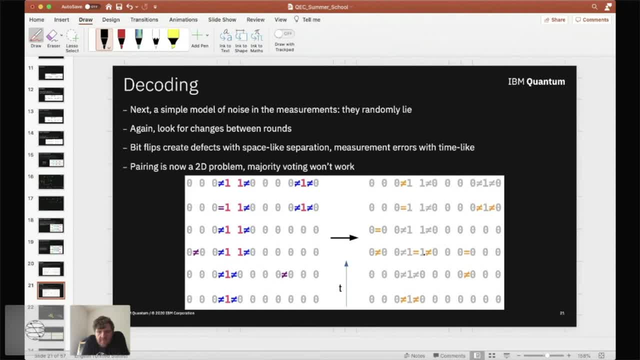 or 0 or 1, can it create a repetition bias? Is such a thing even possible on a quantum computer? A repetition, what, sir? A bias? Well, yeah, so I'm not really sure actually of what's being said. 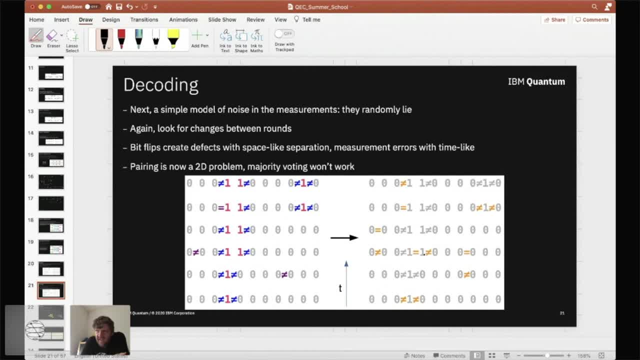 It will cause problems if you do everything by repetition. So I think we should speed on to the surface code and show how things are really done in quantum error correction. But trying to explain decoding in terms of that first would have been harder. But let's finish off with the repetition code. 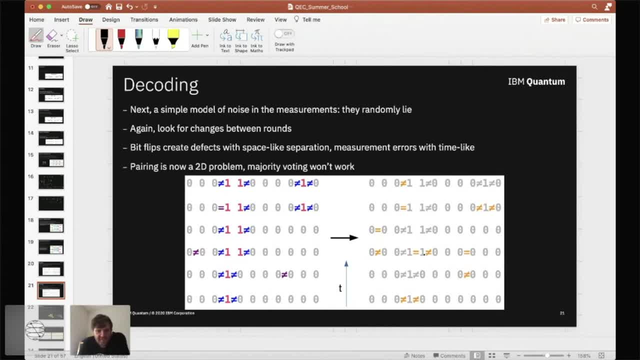 and then we will get on to proper fontanara correction with the surface key. great, and just one last thing, james, if you don't mind clicking the red pen instead of the black one. people in the chat were saying it would be easier to follow the red pointer instead of the black one. oh, maybe even highlighter. yeah, good idea, okay. 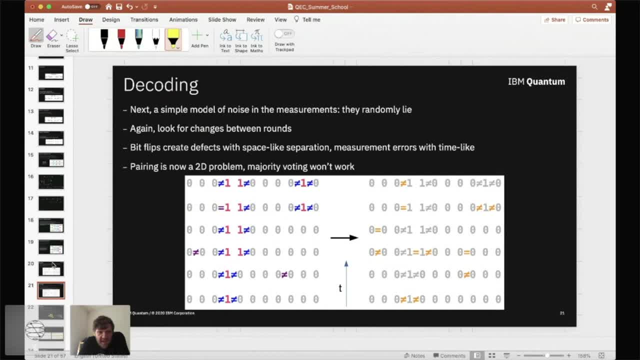 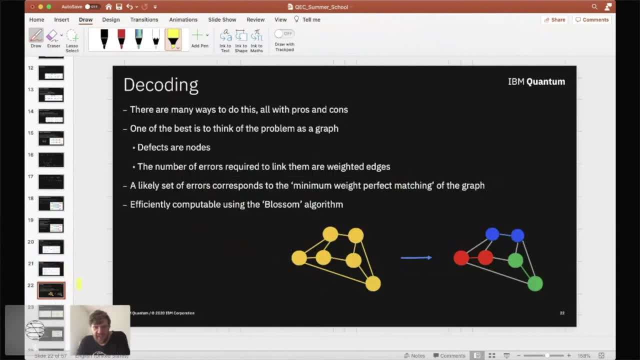 thanks, so, um yeah, so this gives you a sense of fontanara correction. but really quantum error of decoding, but decoding something you've got to get your hands dirty with really, um yeah, so also one sort of one thing to note is that we- we usually do this by graph, theoretic. 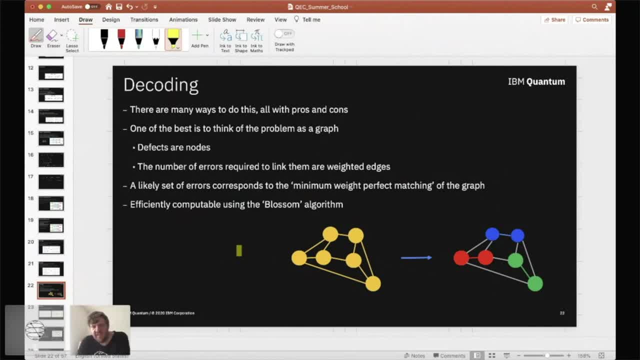 algorithm. so some, if any of you know about graph theory, then you will be especially adept at um grasping some of the concepts in quantum error correction. uh, typically we use something called minimum weight perfect matching um, but uh, i love the quantum error of decoding and i think there's a lot of people who don't know about quantum error. 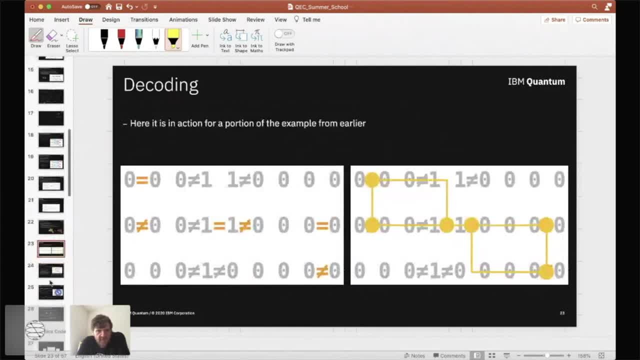 so i think there's a lot of people who don't know about quantum error, so i think there's any real need to go into any details on that, and so let's um, so, let's move on. oh, so one thing, let's actually look at an actual example. so if we had this set of errors, what would we assume happens? 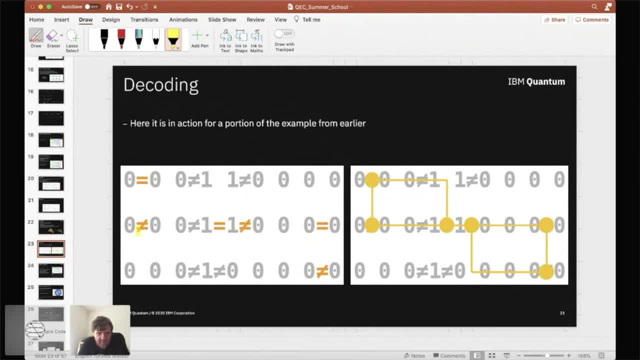 well, we can see that here's a pair of weird things, so probably that means that this was an error. here's an error here and here and here, flipping these three, and that's what caused a couple of things to flag up here, and similarly, errors here, here and here, and this is less likely because there's more. 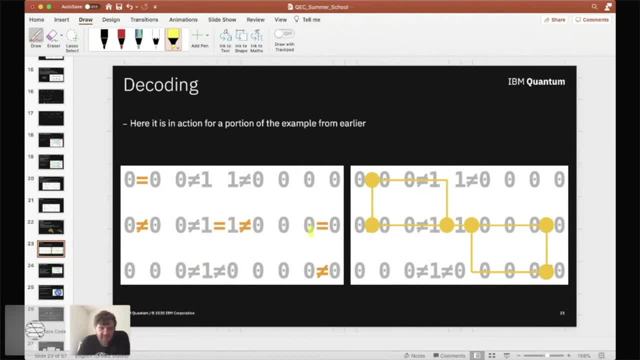 errors, and so we're really comparing different possibility, possible things that could have led to this happening, and then trying to minimize and find the most likely. so this is what we do by the algorithms, and there's there's various algorithms that can be used to do that. so 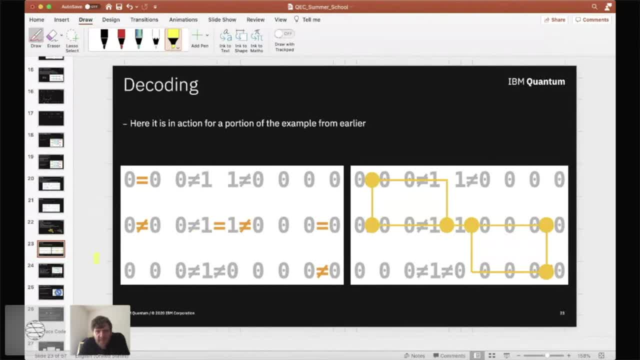 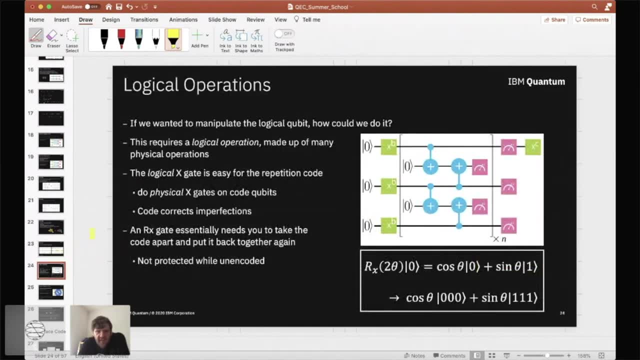 let's look at a couple of examples here. algorithms, um, but yeah, i think i'll. i'll move on and let you look into those in a bit more detail. okay, let's talk about logical operations. if we did not just want our qubit to sit there and be zero or one, but we actually wanted to do things to it. 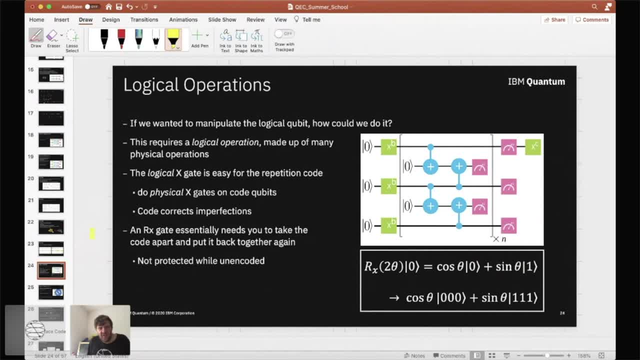 how would we do that? so this is the notion of a logical operation. so when we encode in quantum error correction, we take a single qubit of information and spread it across many qubits. similarly, when we want to do something to that, if we want to do an x operation on our qubit, we 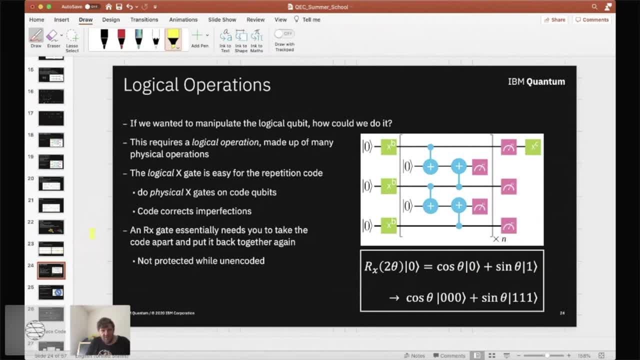 cannot just do it on a single qubit. we have to do it across our entire encoding in some way, and the way that we do this depends on the exact code that we're using. um. so for the, for the repetition codes, flipping the bit is quite easy, because we're just repeating zero. 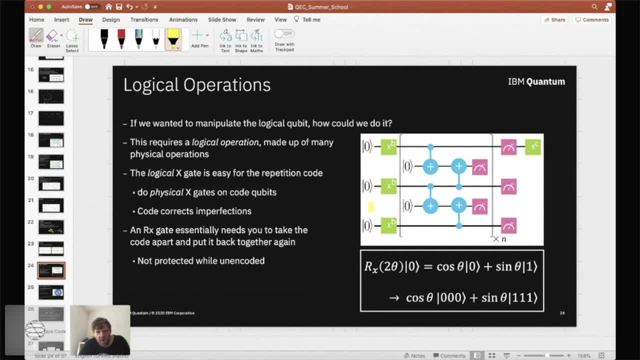 zero, zero, or we're repeating one one one. uh. so if we want to flip that bit, all we need to do is flip everything. we flip all of our zeros to ones, or all of our ones to zeros. so at any point between a couple pair of these measurement rounds, we can just flip all of these qubits, and that would be. 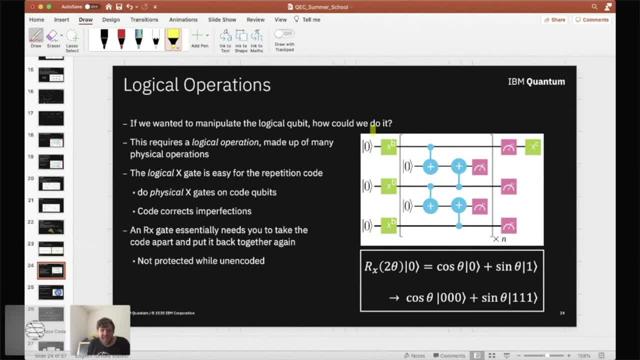 that would. so we can do an x on all of these qubits and that would do a logical x. it would do an x on our encoded information, and the nice thing about this is that when we do a logical operation on our encoded information- and the nice thing about this is if these were a little bit imperfect- 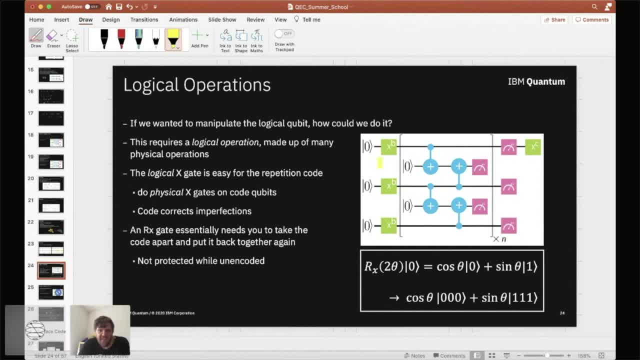 then, uh, that it would also. that would just effectively be the same as if we did them perfectly and then followed that up with a little error. and but we, as we know, errors that occur between measurement rounds are pretty easy to correct, so we would not just be doing. 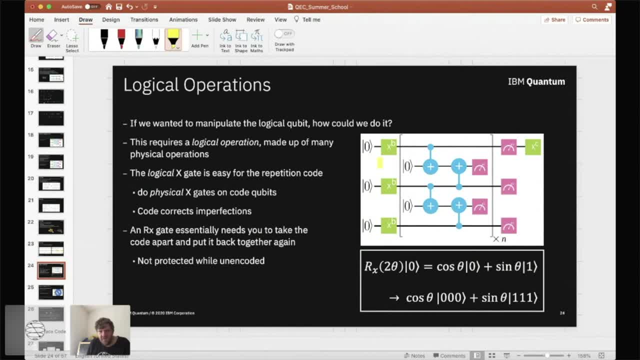 a x operation on our encoded information, on our logical information. but also any perfections in the way that we perform that operation are removed by the same error correction process, which is keeping the qubit clean. so this is a logical operation, it is a perfect operation on our perfect qubit, which is awesome. um so doing an x gate on the repetition. 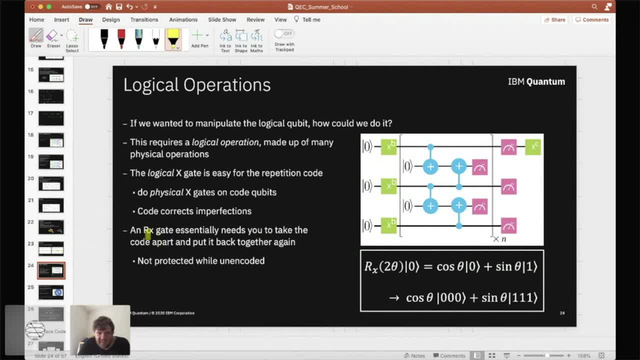 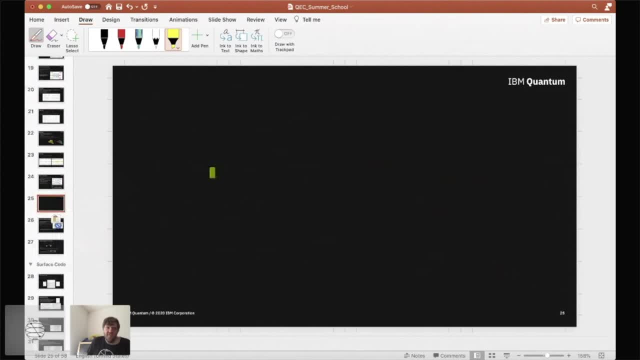 code is easy, but what if we were to do, say, an rx gate? so what would an rx gate mean? it would mean that we want to um, not just so. an x gate means that if we have a zero, we want it to become a one, and we're doing that by turning the zero, zero, zero of our repeated encoding. 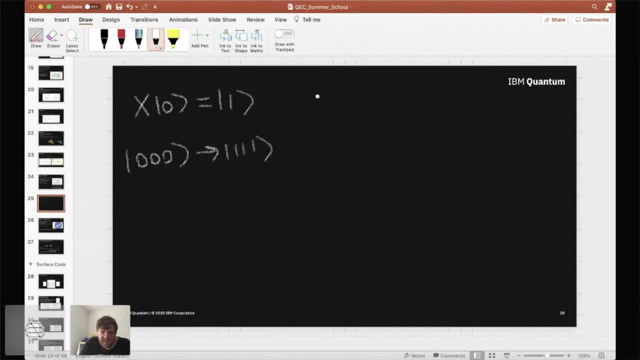 into one one one. uh, an x gate similarly means that if we have a one, we want it to become a zero. so it means that we're turning our one one one into zero, zero, zero. and we just do that using an x, x, x if we're doing three repetitions at least, but an rx gate or any other single qubit. 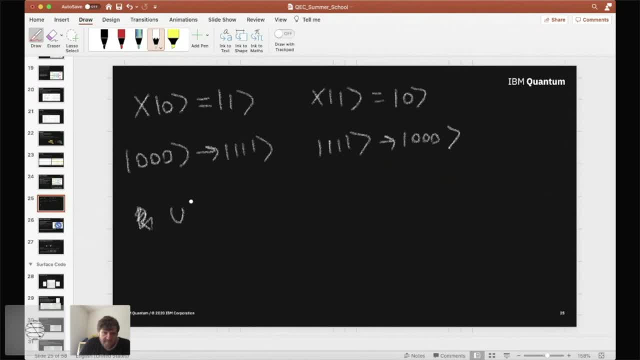 rotation, in fact. so let's just say a? u, any single qubit rotation would take zero and make it to some general superposition of zero and one. so in an encoded form that would mean that the logical version of this has to take zero, zero, zero and turn it into some sort of a zero, zero, zero plus b. 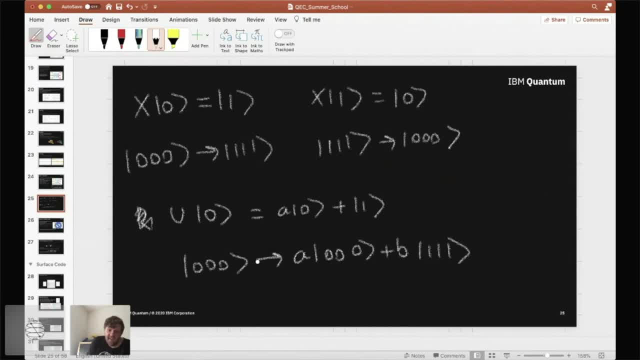 one, one one. now, this is an entangled state. the only way you can make an entangled state is by using control two qubit operations, such as controlled knots. so already just by looking at the state we know that it's not going to be as easy. here we could make an x. our logical x was just x on the three qubits. 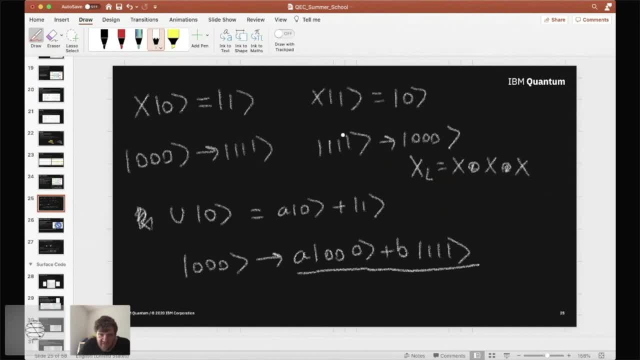 so this x tends to productive with x tends to productive with x. i've written there: we would hope that our logical u might just be similarly, that we do the u three times. but unfortunately that is not the case, because we can see here the fact that it is entangled. it obviously needs some controlled. 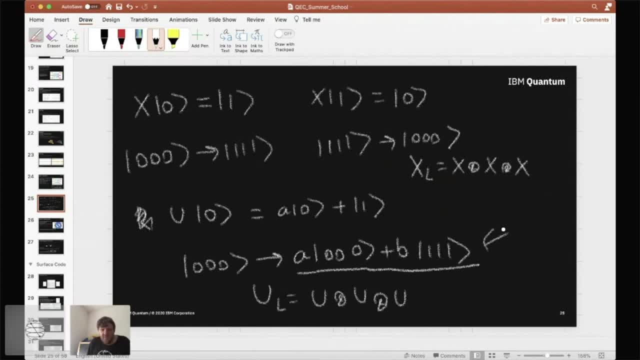 knots in some way. and if you look at it in more detail, what you find is basically all we can do is take our encoded information and unencode it so that our logical qubit just sits on one physical qubit. then we do the single qubit rotation and then we re-encode it again. 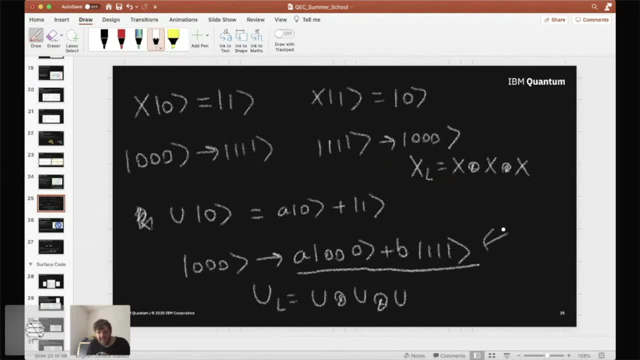 again. but in that whole time that it is unencoded, just sitting there on a single physical qubit, it is exposed, it is no longer encoded, it's no longer having error correction done. any noise that happens then is noise that cannot be undone. any noise, any imperfection in this u-gate that we 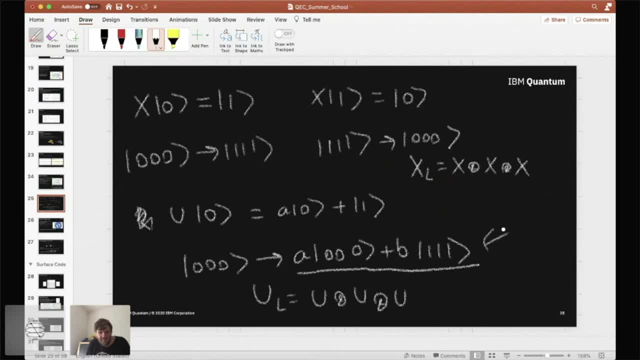 are performing just sits there, it happens. it cannot be undone um, so you cannot fault. tolerantly do any arbitrary single qubit gate using the repetition code, and that is bad, because we need to do those things in order to do quantum computation um also. so this is a major problem. 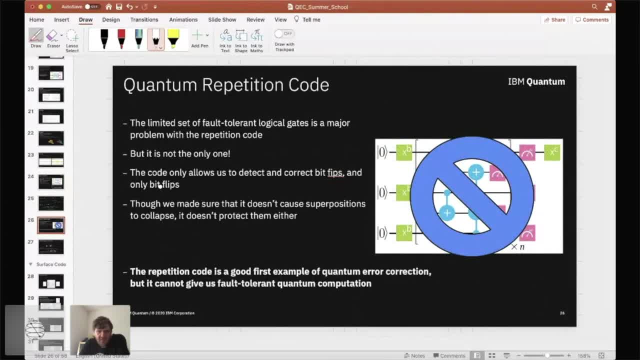 with the repetition code, but it's not the only one. the code only allows us to detect bit flips a lot. it imagines the only error that happens in a quantum system is flipping bits, but that is not the case. uh, there are other things. so a bit flip is basically like an x, like a, an x gate. 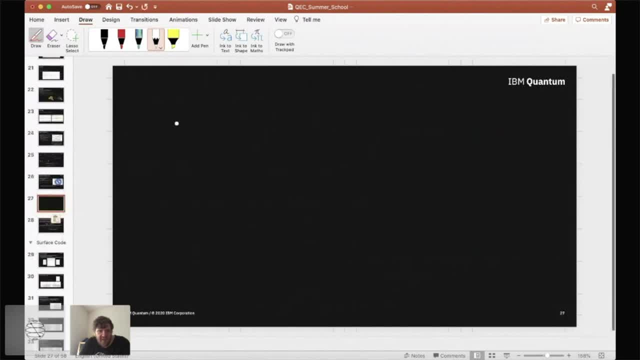 so we're imagining that the only thing that ever happens is a gremlin sits next to our qubits and, with some probability, px hits them with a hammer that does an x gate. that is our error model at the moment. it is a terrible error model. that is not how physics works. at the very least we should have that the gremlin is also able to. 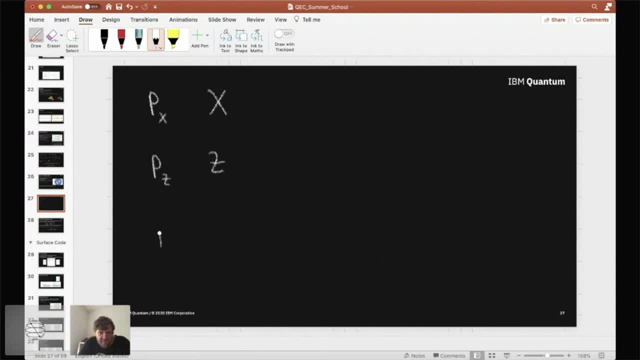 sit there and, with some probability, do a, z and with some probability, do a y, um. in those cases, at least, we would capture something, something more complete. uh, if we had such errors in the repetition code, they this: these errors would not be picked up at all. these errors would be picked up to an extent because 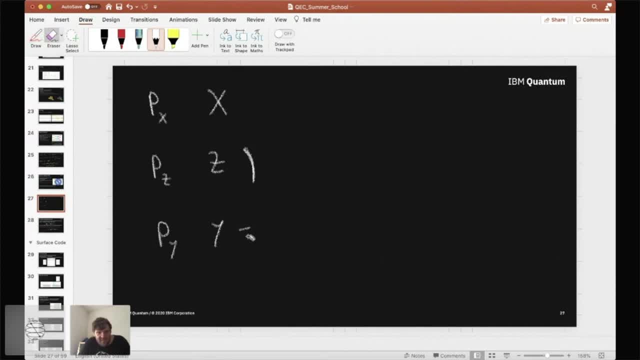 well, because y is, uh, equivalent to um, a combination of x and z, so it picks up the x part but the z part, nothing happens. so if you have some a zero, zero, zero plus b, one, one one, and your repetition code looks at this and says, okay, uh, well, uh, these are the same, that's good. 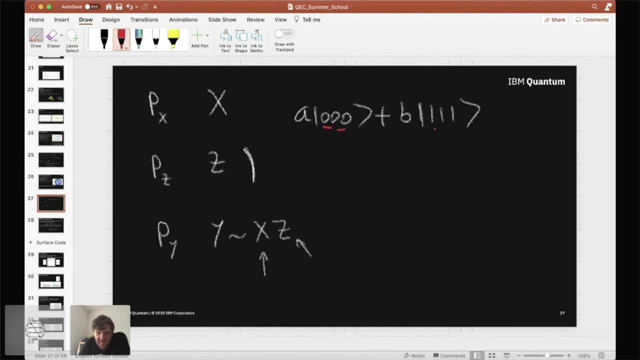 and these are the same, and we would talk to them about Jacqui, about this. so, taking a look at this, these are the same. That's good. Or, in superposition, it's equivalently saying that these are the same as well. It says that everything is fine with this. However, if errors came along and 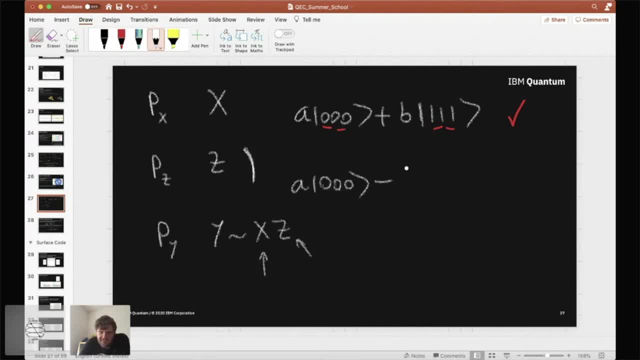 transformed it into the state A000 minus B11, your repetition encoding would come along then and look at these things and say, yeah, yeah, yeah, yeah. Well, good, It would not see this. The repetition syndrome measurements are not set up so that they can see any changes. 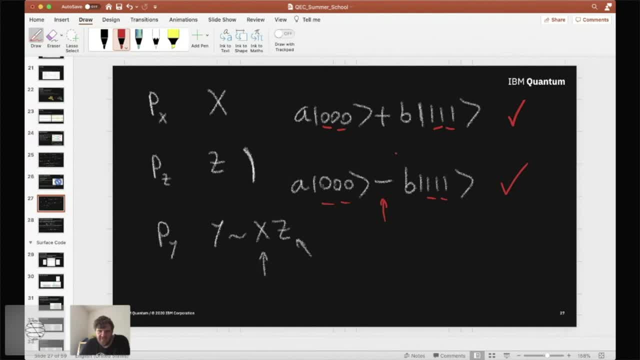 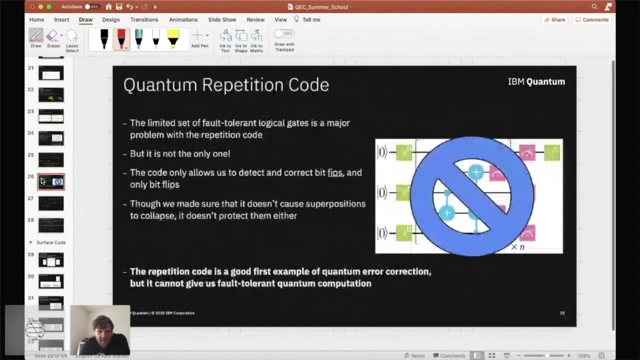 in phase in the superposition. However, changes in phase in the superposition are actually quite big changes and we don't want them to happen. So the repetition code is not the world's best quantum error correction code, And for that reason we have to. So it's. 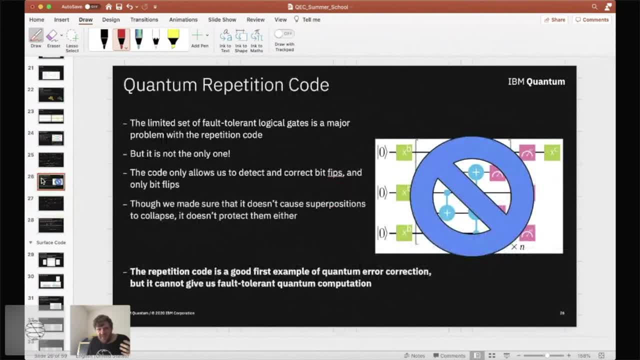 a good first example of quantum error correction. It's a good example of syndrome measurements and decoding, And that's why I think the repetition code is going to be very important for us over the next few years as we test out the capabilities of new devices and see if they are indeed. 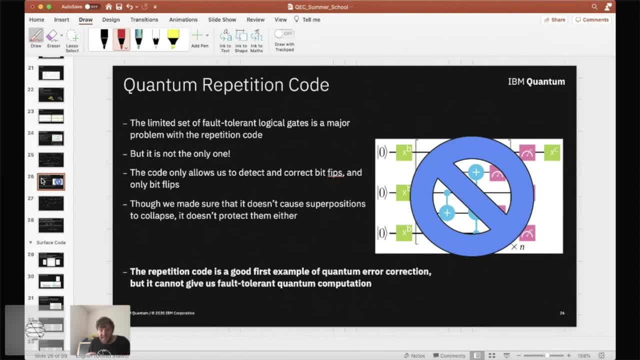 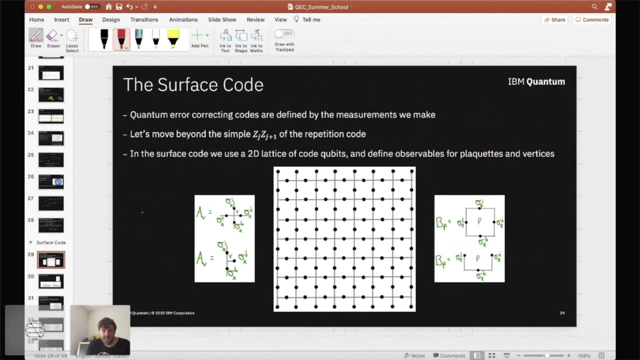 compatible with the needs of quantum error correction, But when it comes to actual quantum computing, we will not be using the repetition code. So let's just move on to what we will most likely be using, which is the surface code. So the surface code is in some ways a generalization of the repetition code. There are things that 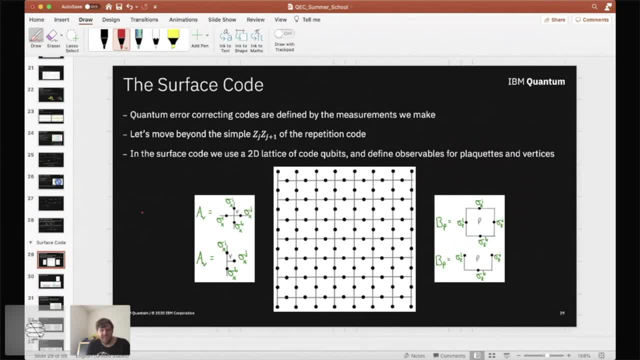 happen in the repetition code, which happen in very similar ways in the surface code, but it generalizes it to make it Well solve the problems of the repetition code. So the noise is no longer just going to be about bit flips, It's going to be a more general. 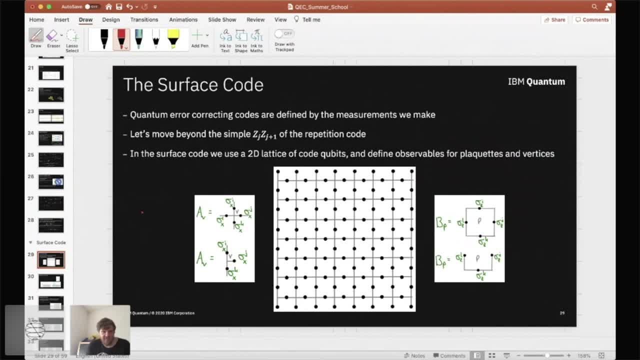 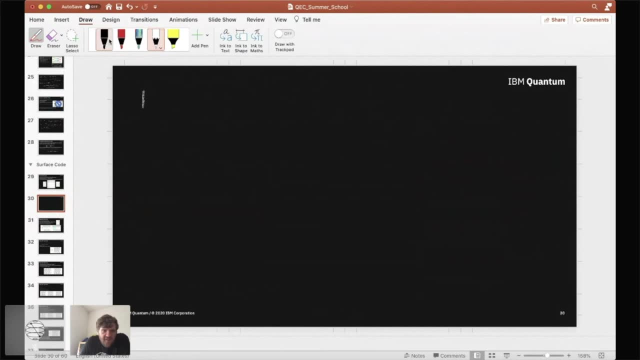 form of noise and we are going to be able to determine that, Okay, Okay, So for this we need a new type of syndrome measurement, And so in the surface code we use- Sorry- in the repetition code we use these syndrome measurements where we have. 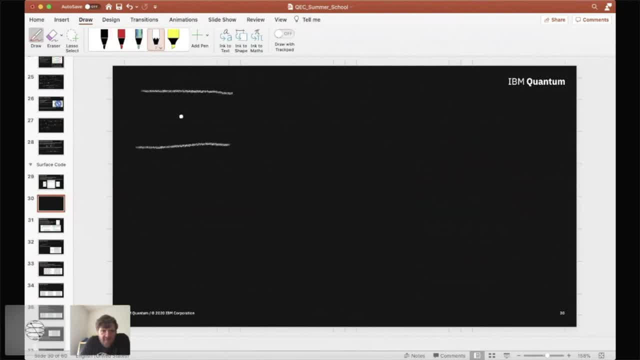 a couple of qubits from our code and they're being joined by an extra qubit and we have some CNOTs going on and we have a measurement at the end. It looks like the Enterprise. I never noticed that before. 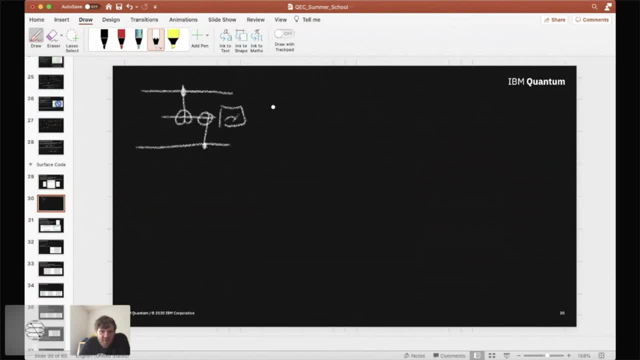 Yeah, So this is what our syndrome measurement and these qubits in the code carry on their lives. after this information extraction event has gone, which no longer looks so much like the Enterprise, We could also say that what we are doing is measuring the observable z, j, z, j plus 1,. 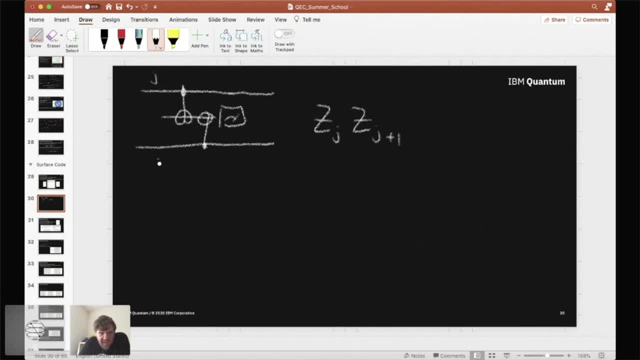 if this is comparing two qubits called j and j plus 1.. Okay, So this is an observable. So let's not get too much into the maths. but z as you'll see if you look into some of the sections in the first couple of chapters of the Qiskit. 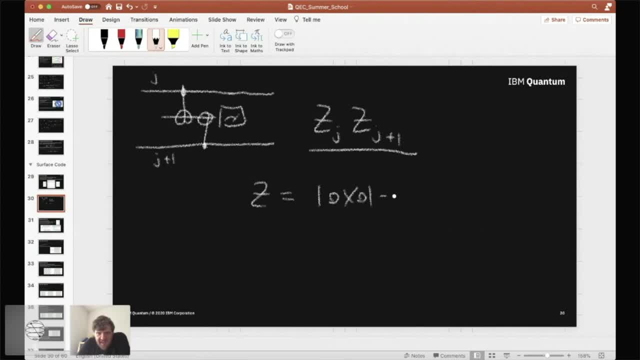 textbook z can be written in this way, So it has, So it's a mate, So it's an operator with eigenstates and eigenvalues, and the eigenstates are 0 and 1, and the eigenvalue for 0 is plus 1, because there's a factor of plus 1 here, and the eigenvalue for 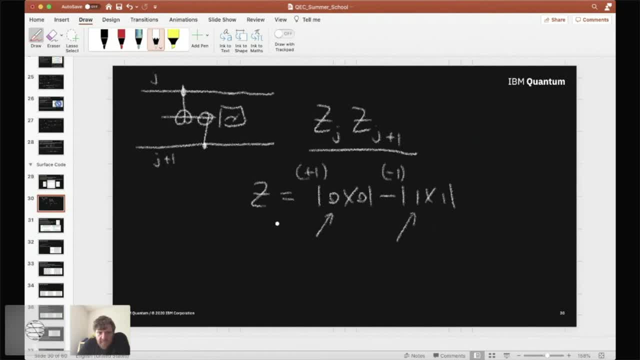 And the 1 value is minus 1, and the fact that these have different eigenvalues is why they give us different results when we measure them. Now, if we were to look at the operator z j, z j plus 1.. 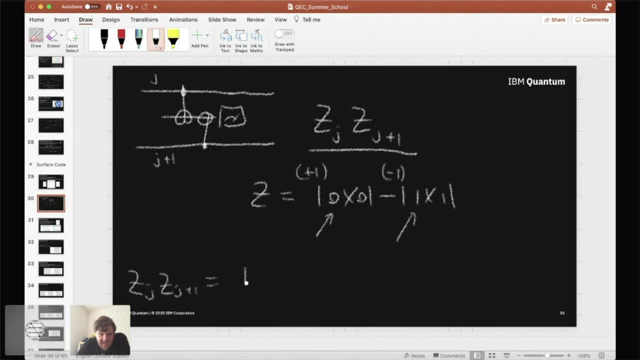 Then this has eigenstates 0, 0, and 1, 1, both, Oops, that's a little bit big. So the 0, 0 and the 1, 1 states 0, 0.. Oh, that's a roller, or an eraser, as I should say. 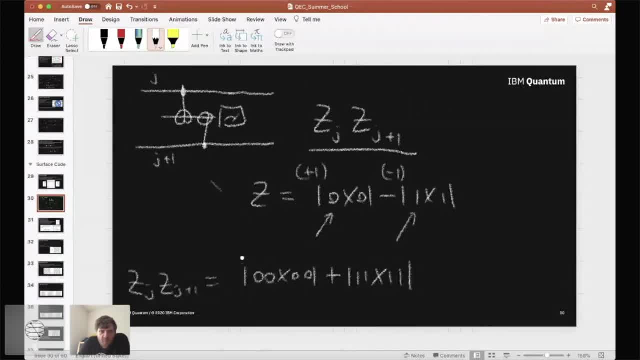 in this more international audience. Okay, Okay. So we have these eigenstates 0, 0, 0, and 1, 1, and then we also have the eigenstates 0, 1, and 1, 0.. 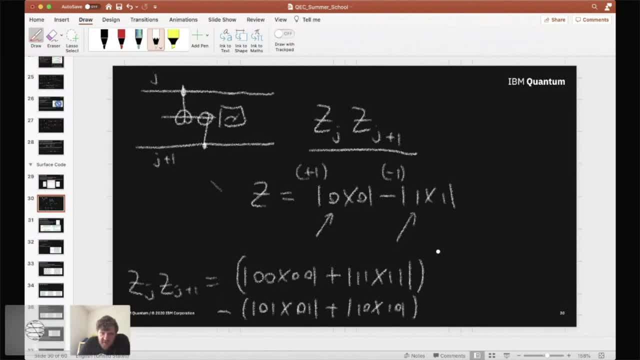 And so these have eigenvalue plus 1, and these have eigenvalue minus 1, and that's why, when we measure this, We get a certain outcome, depending on whether it's one of these states or some superposition of them, and we get the other outcome depending on whether it's one of these states, because 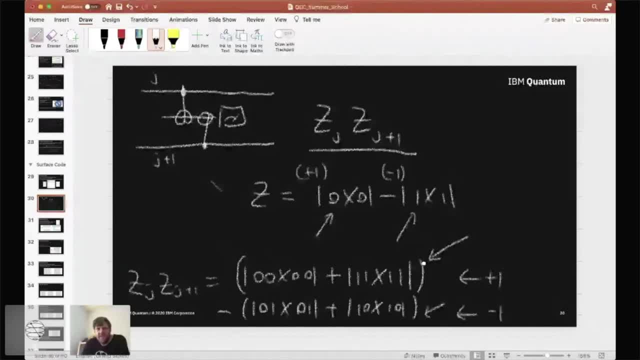 they belong to different eigenstates, So this is the way that we can describe this Now. in other error correcting codes, we usually, instead of writing down the circuit and saying my syndrome measurements look like this and then noting that they could be described as: 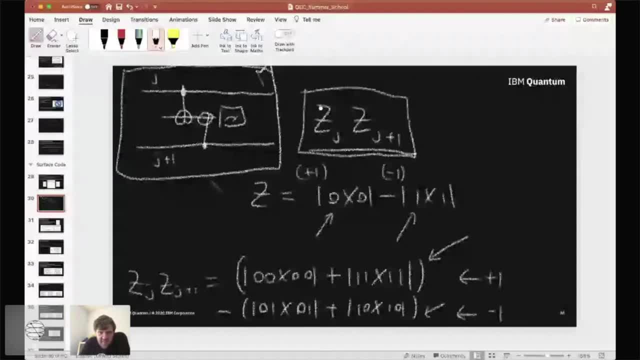 measuring an observable that looks like this. Okay, So let's say, my syndrome measurements correspond to an observable that looks like this, And of course you have to measure them somehow. This circuit seems to work, so let's use that. So usually we state what our syndrome measurements are in terms of observables of this form. 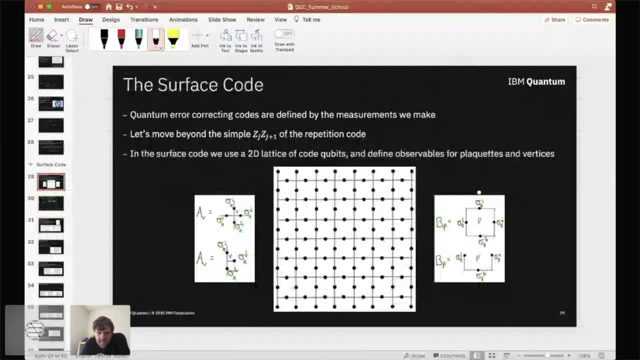 So, for the surface codes, these are what the observables look like. We have a grid of qubits, So all of these things on here are. These are qubits. This is a square lattice of qubits. We arrange our qubits on a square lattice and what do we do? 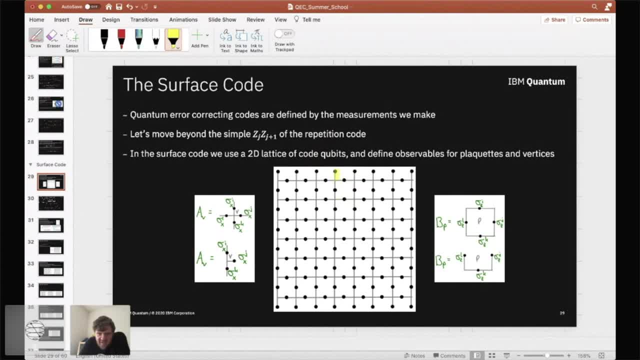 We associate with each of those, for each plaquette, so for each square on the lattice, we associate a type of measurement, a syndrome measurement that we're going to make, And it corresponds to this observable, which is a tensor product of Z operators. 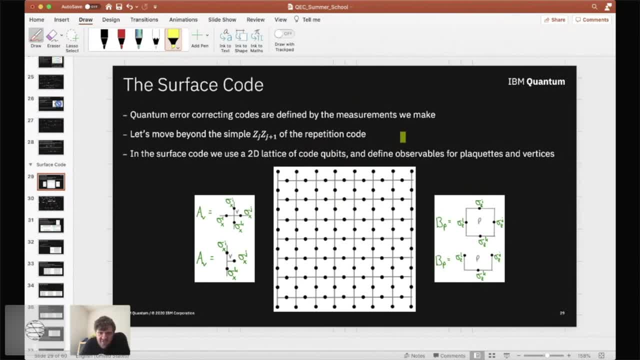 I've written them as sigma Z here rather than just a Z, but often I write sigma Z instead of Z For physical qubits and Zs for logical qubits, but I'm not going to follow that convention completely throughout this. So for every plaquette we associate a type of syndrome measurement, and that's also true. 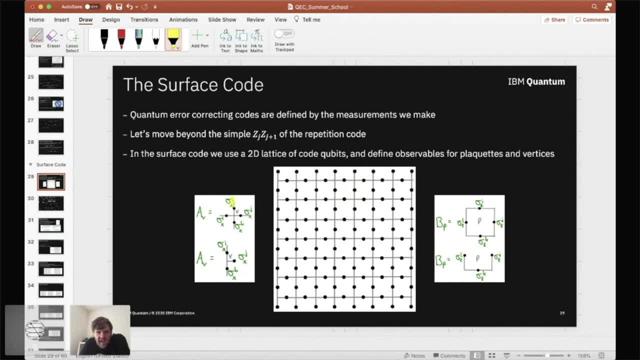 for these sort of truncated plaquettes at the top and the bottom, And for every vertex we associate a different type of measurement, and that's also true for the truncated vertices on the left and the right. And yeah, Okay, So you can look at these and you can think. well, I have no idea what they are saying. 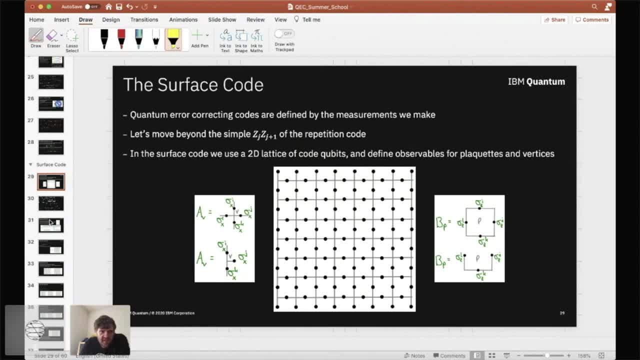 but don't worry, We are going to figure them out. So what we are going to do is we're going to. so the surface code only works if you do the measurements associated with the vertices and the measurements associated with the plaquettes. 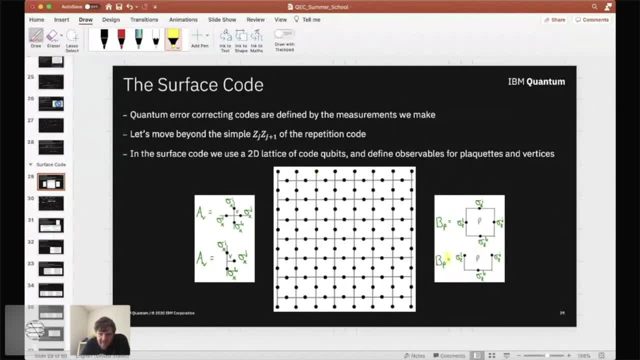 because these are going to pick up on certain types of errors and these are going to pick up on other types of errors And it's only when you put them together that they are going to pick up on everything and be a good quantum error correcting code. 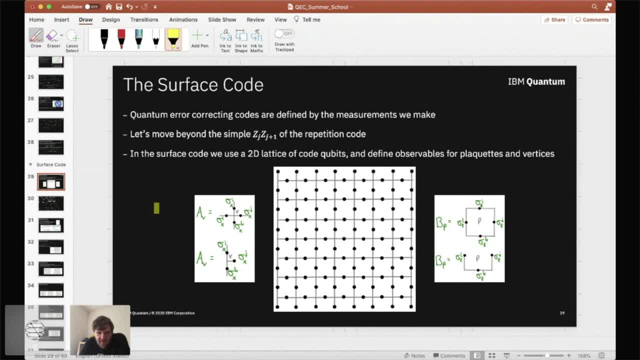 However, the way we're going to try and understand what's going on here, so that we can really see what kind of states are generated when we measure these things, is we're going to imagine a surface code that only has these, this kind of measurements, and we're going 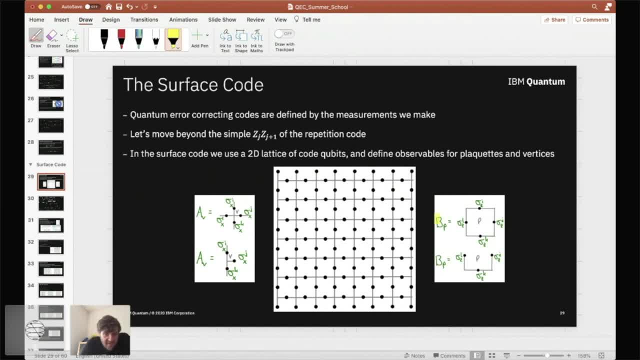 to see what that can be used for. They can't be used to store a qubit, but we're going to look at it anyway. Okay, And then we're going to forget about those and we're going to look at a surface code. 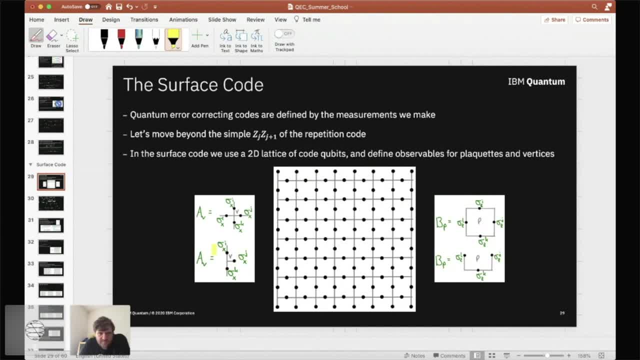 that only has these kinds of measurements, and we're going to think of what that can be used for. And then, once we have looked at these two sort of half surface codes, then we can combine our knowledge back together to think of a surface code which has everything that it. 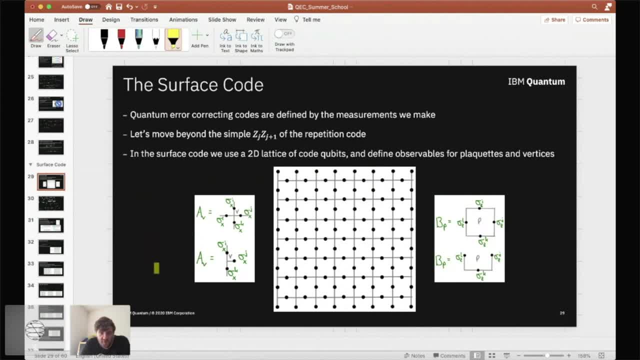 needs and see that this can store a qubit and can store it in a way that is, you know, protected against all sorts of noise. So yeah, actually in a lot of ways, this qubit, this lecture is a bit different in. 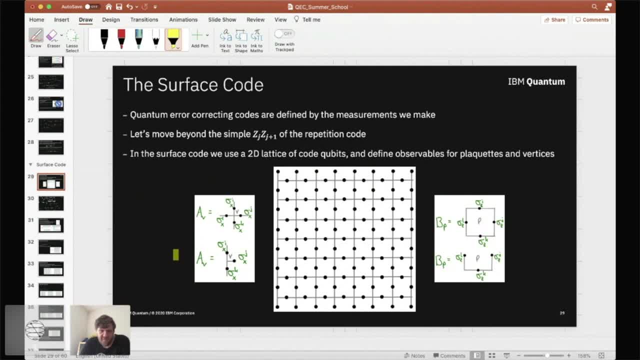 spirit from the previous ones, because at the end of this we're pretty much saying, look, we have one qubit and we can. look, we can do X gates on it and Z gates on it, which is a bit of a letdown after you've learned Shor's algorithm and stuff, but at least this 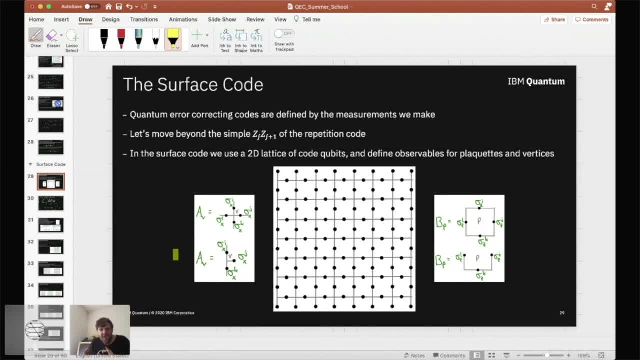 time. our qubit is perfect and we have made it perfect, Okay, But I think it's probably a good idea, since we're coming towards the top of the hour and since I'm going to begin another section, basically that I well, let's do questions. 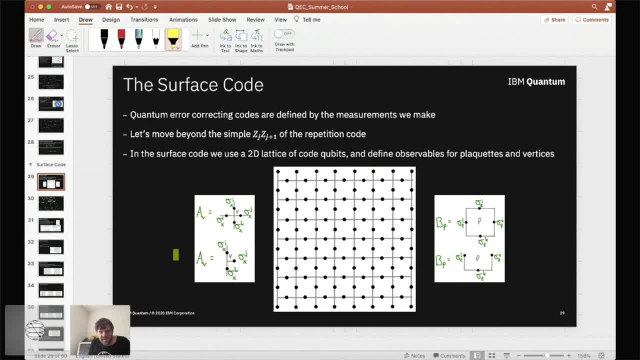 for a few minutes and then let's take another 15-minute break. Sounds great. Again, tons of questions. Thank you everyone. I want to let you know. if any of these questions seem confusing, James, just let me know. 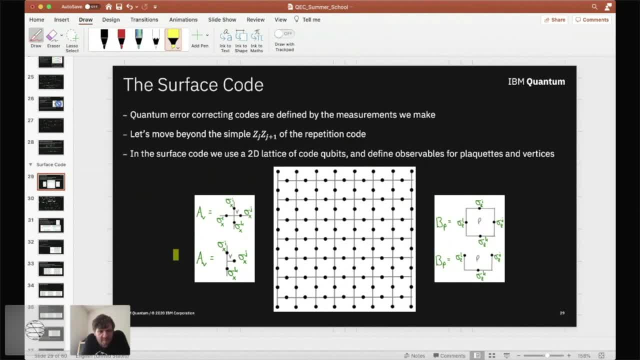 I may be just mispronouncing them, so just let me know. Yeah, Okay, First question: If you see a CNOT gate itself working on the quantum bit, why can't we say the CNOT itself will give some error resulting, even if they are the same. 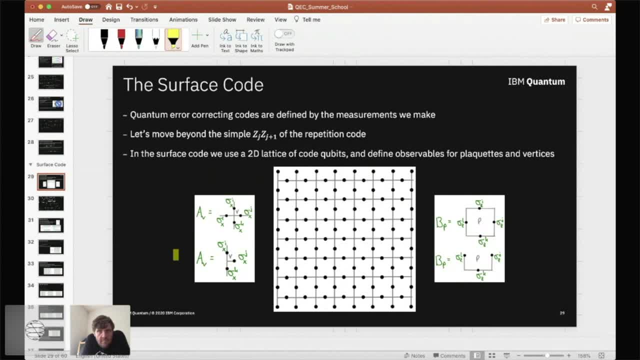 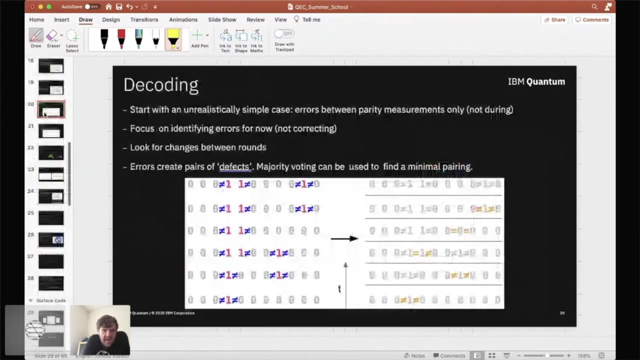 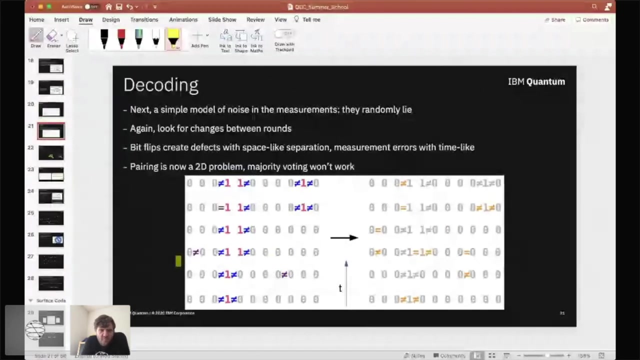 It may give an error, as if they are not the same. So, yeah, it might. So here In the, In the, In the petition code before I covered this thing, that maybe the measurement results lie somewhere over here, And that is a very simple model of how the whole process could go wrong, because it's. 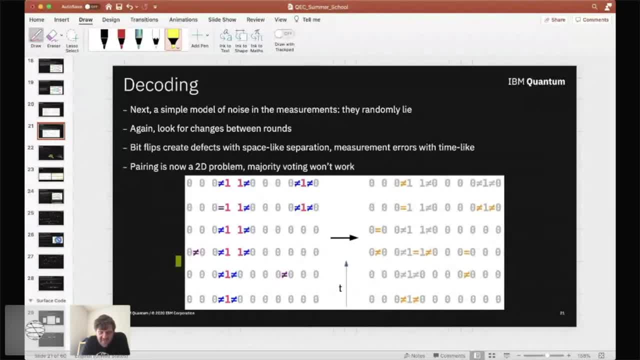 assuming just it lies at the end and nothing actually affected the qubits. Actually, all kinds of things can go wrong and these affect what you see here. So if you look at the syndrome, then you'll see The traces of all kinds of different forms of error, but they all 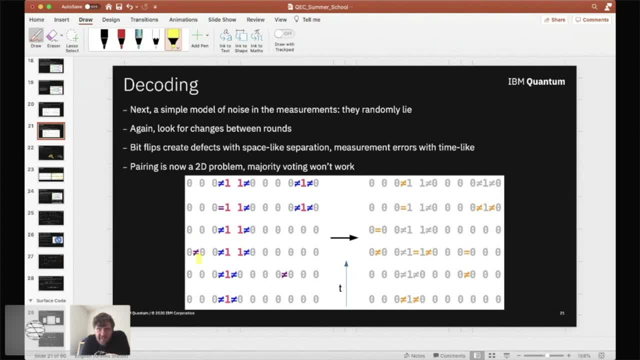 They all. And then you have to make sure you're decoding those that such processes can occur. But yeah, all kinds of things can go wrong, but none of them are disastrous in a well-designed quantum error correcting code. And you have to prove that your error correcting code is well-designed before anyone takes. 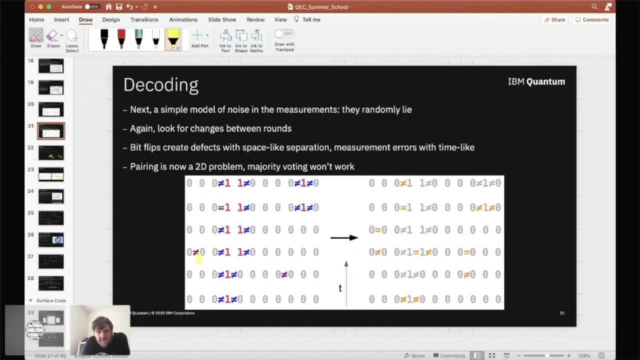 it. Anyone takes it seriously, Awesome. Next question. Next question: we have, and I believe you have, some papers on this. Have there been experimental demonstrations of quantum error correction And if so, maybe after the break could you share some of those references? 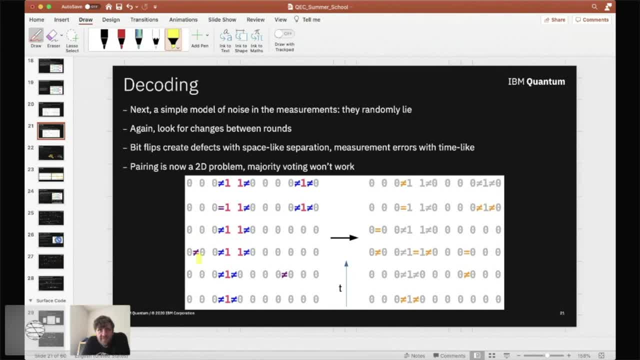 Yeah, So I should try and pull together some references, but that Well, probably the best thing to do is to show off my new paper, in which I do exactly that, Because, Hello, I'm going to show you a picture of a very interesting experiment. 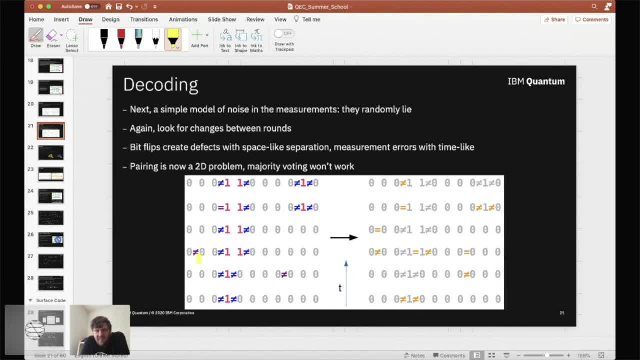 Yeah. So people have done various error correction based experiments, Ones that do syndrome measurements, ones that prepare the state of a bunch of qubits encoded in a quantum way, Some that detect and correct errors in the repetition code. But no one's done the full everything yet. 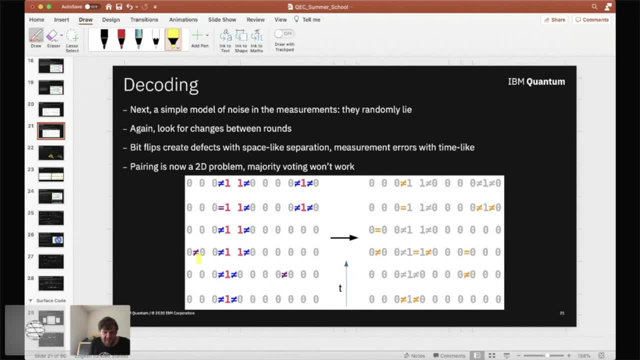 No one's ever combined all of the Yeah aspects as far as I know, Just because you need so many qubits in such particular configurations in order to do that. So the repetition code is great because you can detect and correct things. 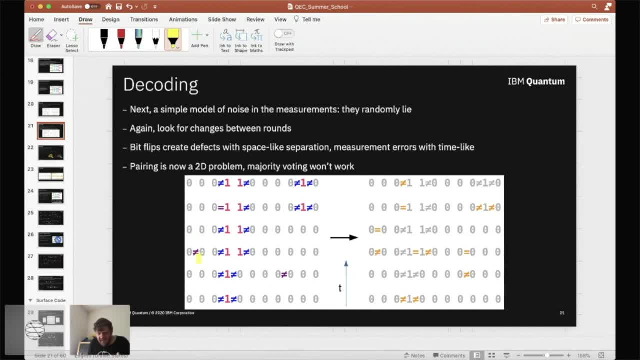 So you can show the whole. Everything the repetition code is you can demonstrate even with current technology, And that's something that's going to be looked at in the lab for those of people who are looking in the lab, But also, I'll share a link to: 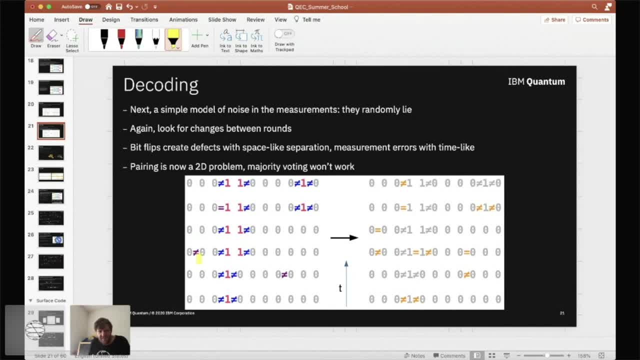 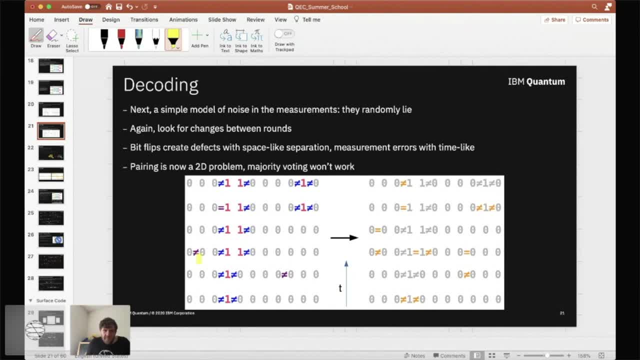 Yeah, Yeah, Yeah, Yeah, Yeah, Yeah. You can also- Now I need to show a link for a paper- Go to the Repetition Code chapter of the Qiskit textbooks, because that tells you how to make a repetition code happen yourself. 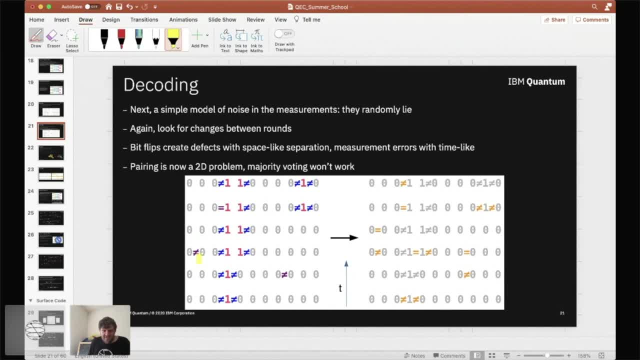 So in terms of experimentantly demonstratingwaldz correction, you could do it today, Awesome. And then one final question is actually another kind of set up here and how it's viewed, and i know you do cover that in your lab, but just wondering if you wanted to. 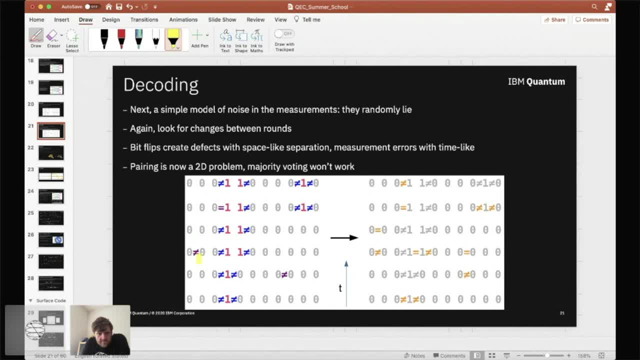 give a quick uh overview of what ignis is here during the lecture. yeah so, um, ignis is is about working out how good devices work. uh, so it can be about characterizing the noise. so you have, uh, something called randomized benchmarking, which is what is used to get all of these numbers. uh, 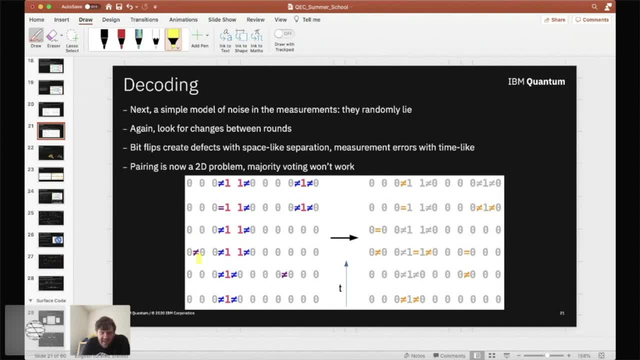 regarding the uh, how good each qubit is and how good the gates are. so you can do your own randomized benchmarking. there's also this concept of quantum volume that we use to be a sort of it's hard to. it's hard to summarize how good a device is in a single number, but it's. it's also something. 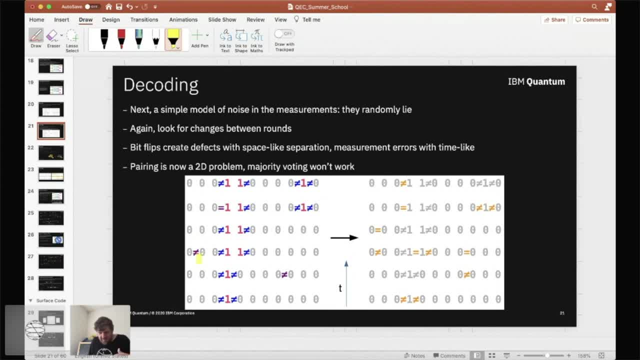 quite useful to be able to do, to be able to describe things quite more simply to people. um, so quantum volume is our way of trying to describe things in a single number, and then that is basically a test which comes up with a score for how good a device is. and so ignis does that as well, and, um, it has quantum error correction. 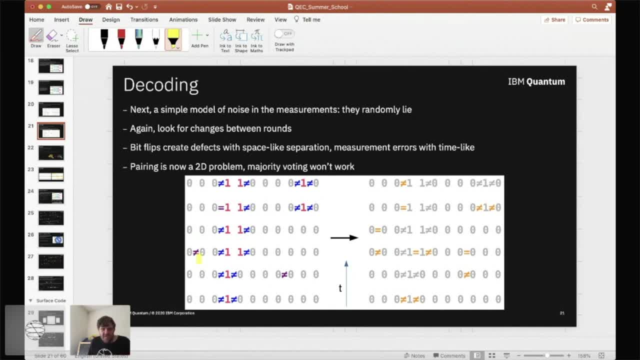 in there, but quantum error creation as a test. you you run it to be able to see how good your device is. so, um, yeah, ignis is mostly all about um, ways to test quantum computers, ways to validate they really are quantum computers. but it also does have measurement error mitigation in there, which is 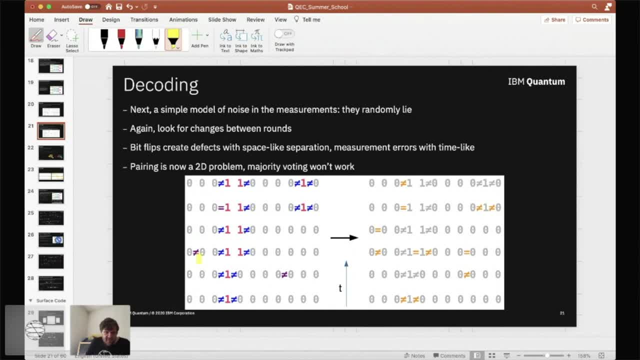 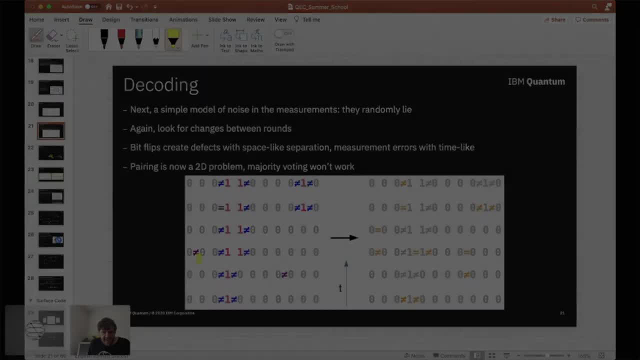 you might want to use in actual applications. it's something you can throw in at the end to clean up the results, basically, and it's, it's, it's. it's almost magical how much you can clean it.